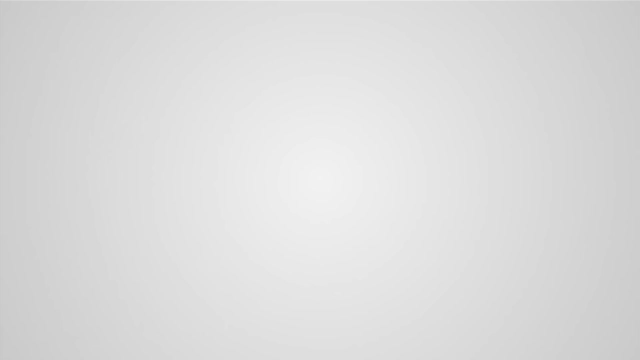 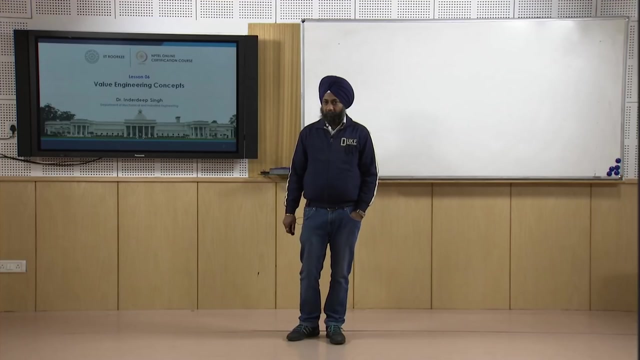 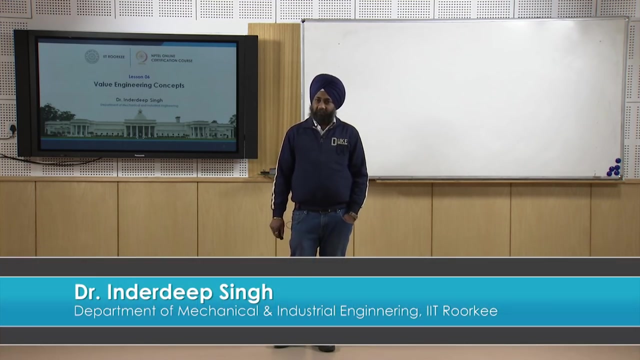 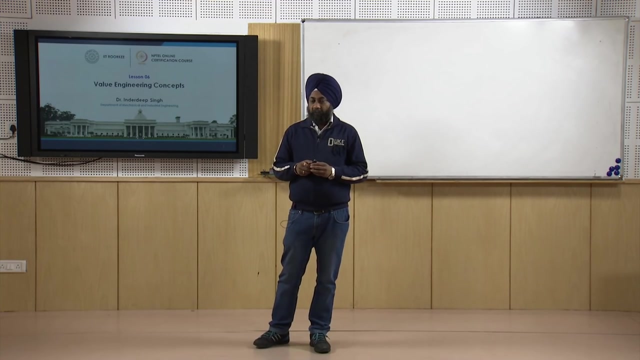 Namaskar, welcome to the second week of our course on product design and development. friends, let us take a brief review of what we have covered in the week one. if you remember, we have covered all the basic aspects of product design and development in week one. we have 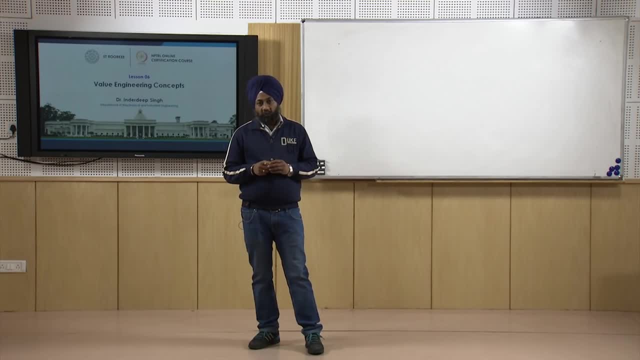 seen what is the need of developing a new product. we have seen the life cycle of a product when it is launched into the market. we have seen the various stages of product development. we have also seen the the product analysis that what are the various characteristics that we need to cover prior? 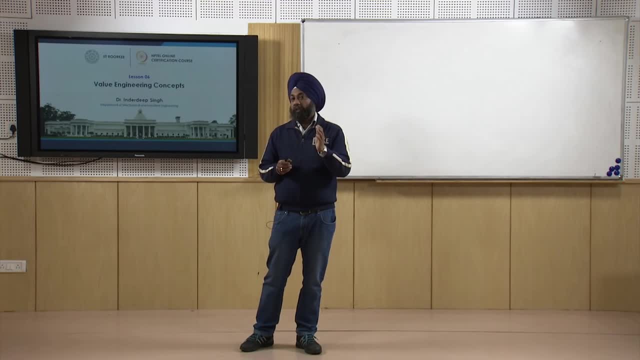 to that. we have also covered that- what should be the product policy of an organization? even we have covered the swot analysis, that is, strength, weakness, opportunities and threats, and the discussion was focused more on the product design aspects of swot. otherwise, swot can be used in all different domains. 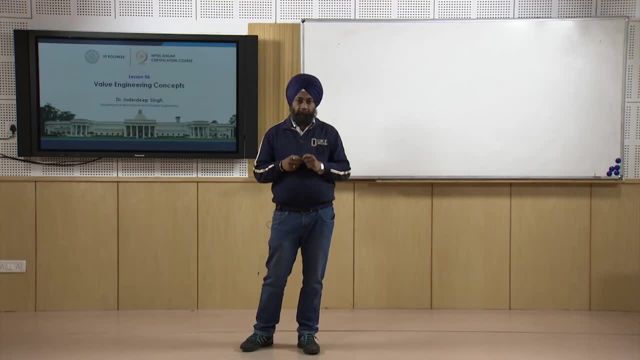 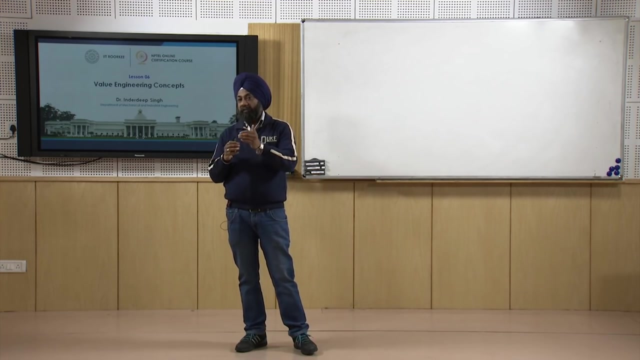 but our focus, if you remember, was on product design, that how swot can be used for product design and in order to launch a successful product in the market. so we have ah build up ah specific knowledge related to product design in our previous week, linking the previous week with our discussion this week. we will see that how the concept 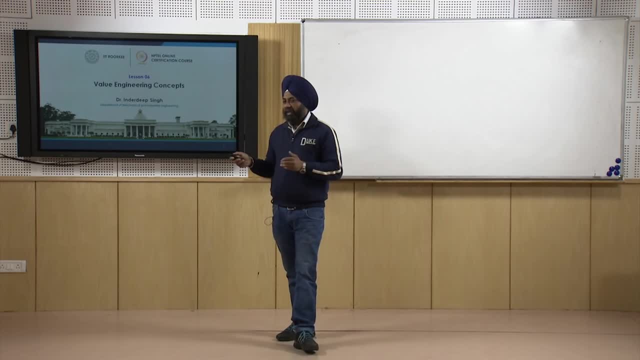 of value engineering, as is clear on собि엔 Ґาո on your slide, are applicable to product design. let me go back again to the last lecture that we had, in which we have seen product analysis in product analysis, if you remember there. 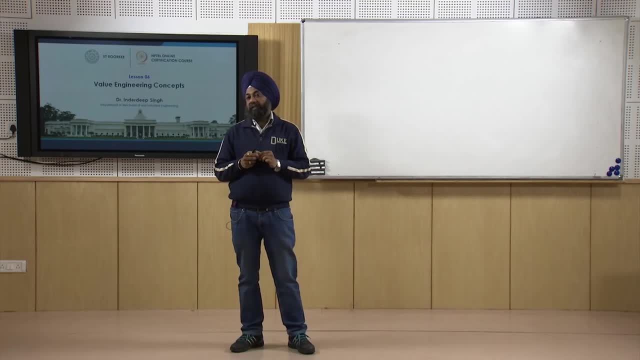 are four broad factors that are needed to be understood, or that we need to understand, in order to design a good, profitable, successful product. if you remember we have seen, first were the marketing aspects. second were the product characteristics. third, if you remember, the economic analysis in which we have seen the break even analysis. and the fourth were 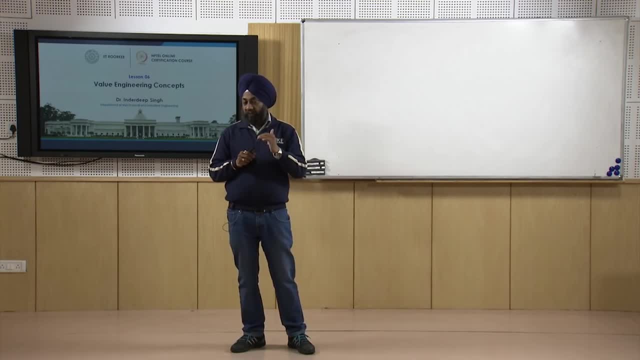 the production aspects. so currently our discussion on value engineering is related to the second important factor, that is, the product characteristics. in product characteristics we have seen that there are functional aspects, then durability and dependability. we have seen the aesthetic aspects. so all these things are required to be understood if we want to develop a successful product. 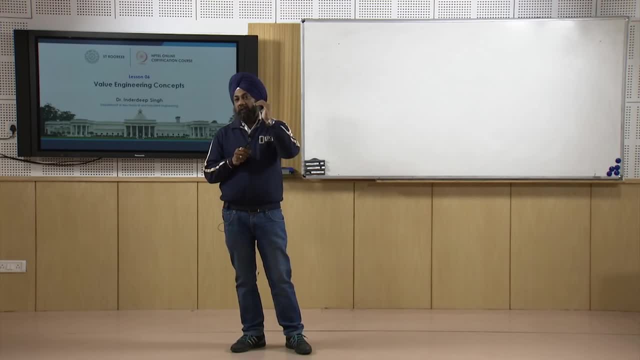 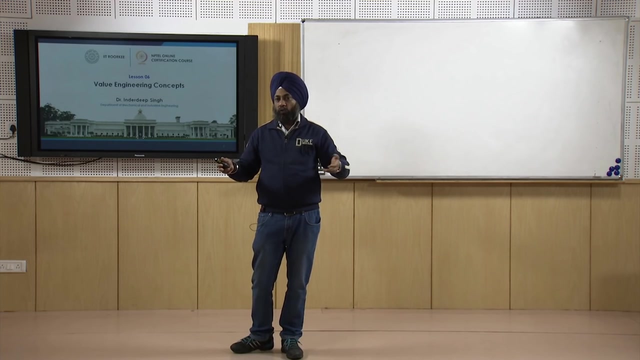 now let us see the functional aspects in product characteristics first. we have seen that there are functional aspects that are needed to be understood. now thing is the functional aspect. so if you see, just free your mind and think that any product around you, in your room or in your classroom or wherever you are listening to this particular 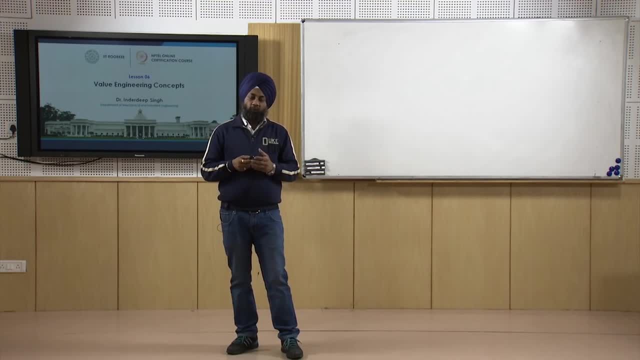 discussion. see any product, why that product has been bought, either by you or by your parents or by the organization. for example, you see a air conditioner. why the air conditioner has been bought: to cool the environment. so what is the function- basic function- of the air conditioner that is cooling the environment. similarly, why i am using this pointer or this. 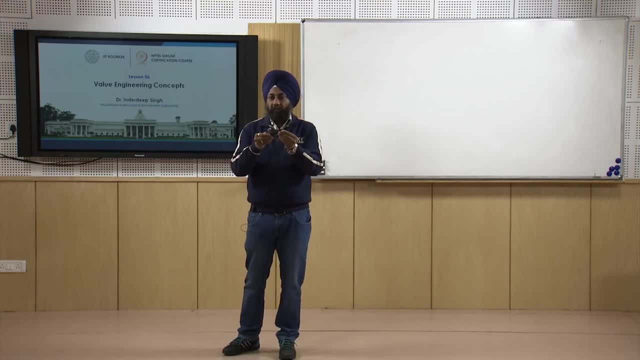 slide changer. it has got some function. therefore, i am using it. similarly, why i am wearing this jacket: ok, it is january going on. there is so much of cold all around the environment. the temperatures are low. in order to protect my body, i am using a jacket, so any product that you see around, 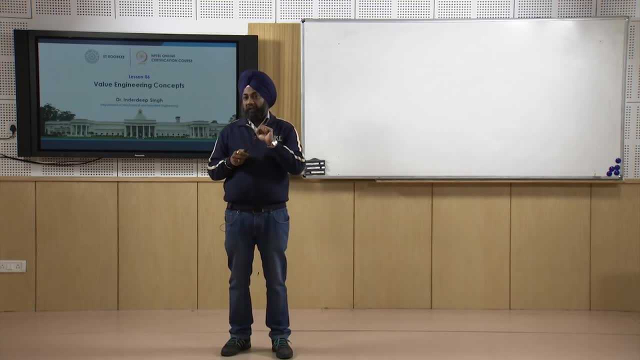 you will have definitely have a function and it will have a functional value and that function has to be provided by that product. and who has to ensure that that the function is being provided by the product or not? the product designer has to ensure that the product is. 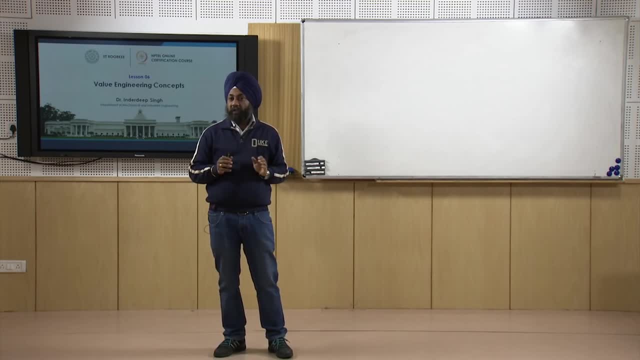 designed in such a way that it satisfies its functional requirement or the functional property for which the product has been designed. i think it is clear to all of you that for any product to be successful, it should be able to satisfy the intended function for which it has been designed. that also satisfactorily and reliably. if the product is not able to satisfy its intended function reliably, definitely that product is not going to succeed in the market. so first and foremost, when we analyze the characteristics of the product, we have to keep a focus on the functional. 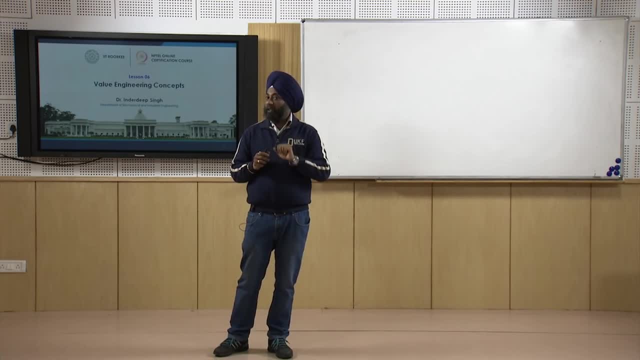 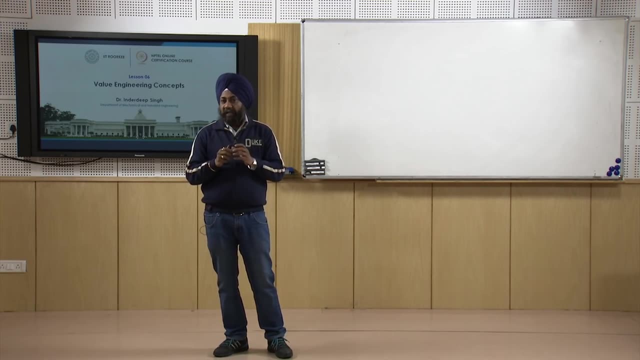 aspects of the product, and for those functional aspects only, we have a concept called value engineering, which is a function based technique and which helps us to ensure that the product performs its desired function reliably, but simultaneously ensuring that this function is achieved at the minimum possible cost. so we will see that what is the concept of value engineering and how it is different. 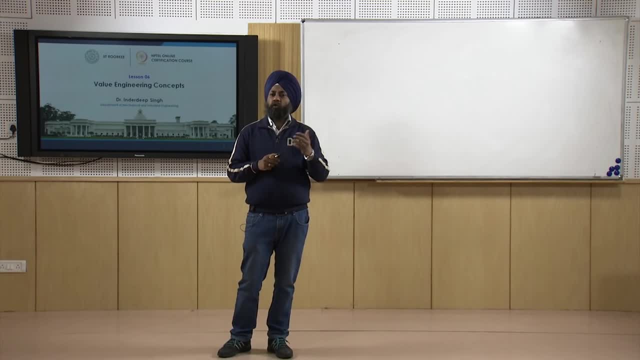 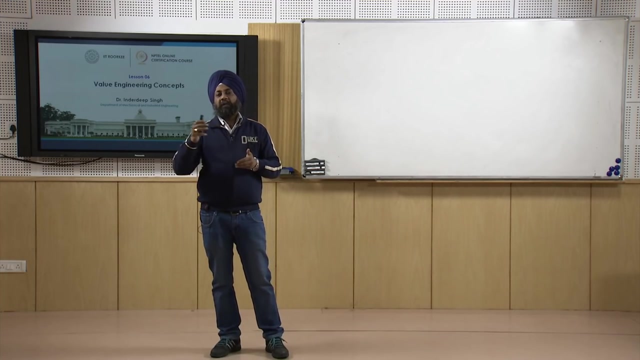 from other commonly used techniques, like cost cutting and the other techniques, like value techniques, of saving money. in this case, we will not compromise on the performance, reliability, quality, efficiency- any of the parameters will not be compromised, but our focus will be to use the systematic approach to cut the cost or to reduce the cost, satisfying all other. 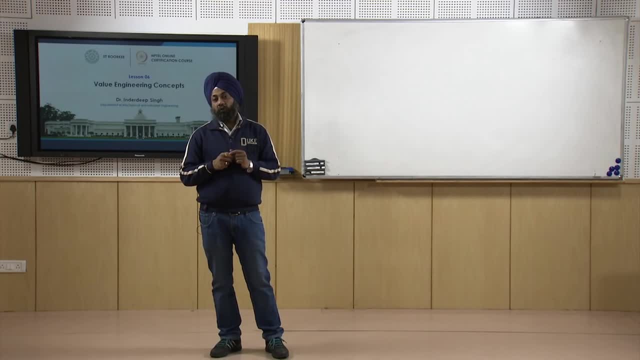 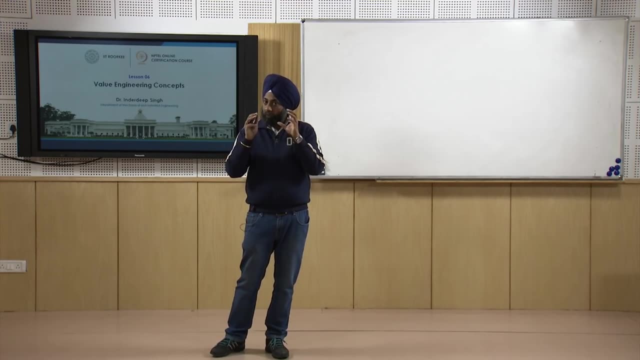 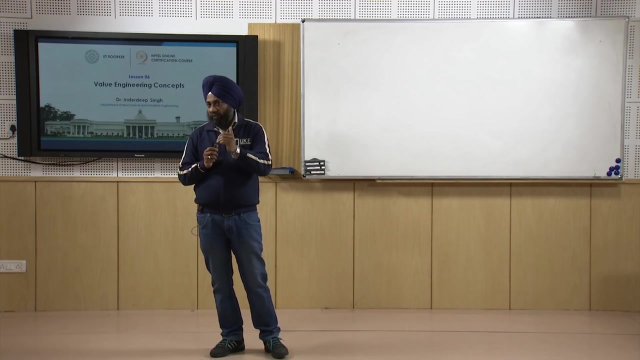 requirements as desired by the product or as desired by the desired from the product by the customer. so our focus will be to ensure this particular aspect of the product. so let us now see one by one, slowly, let us try to understand. this week, our focus primarily will: 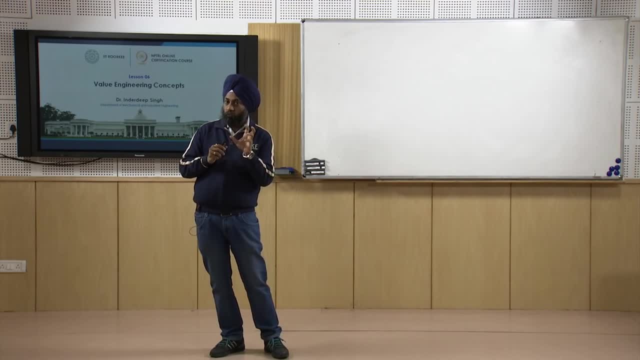 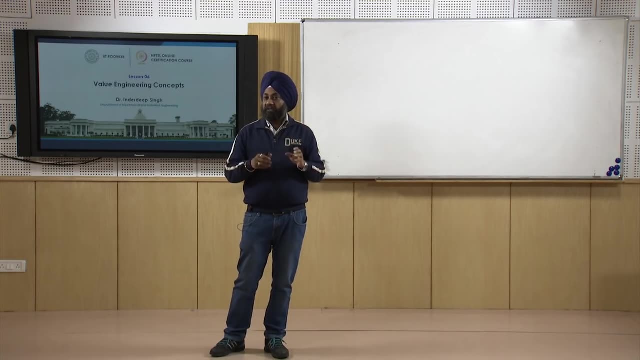 be on the concepts as well as the successful case studies of value engineering. it has been applied worldwide and there are so many success stories where the concept of value engineering has helped people to design the products, to launch the products in such a way that they have been 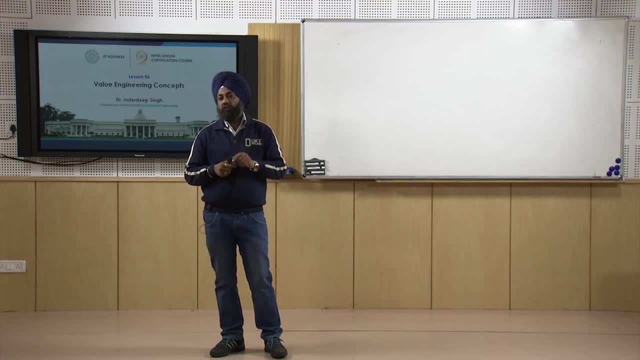 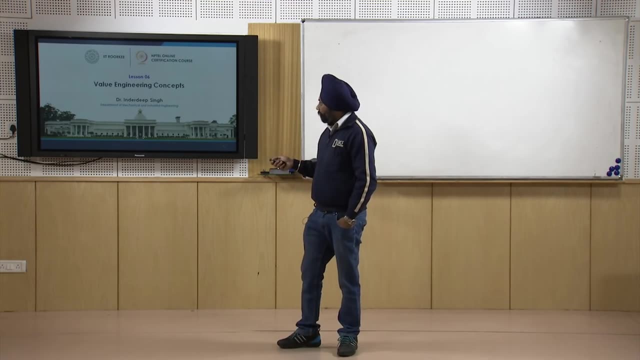 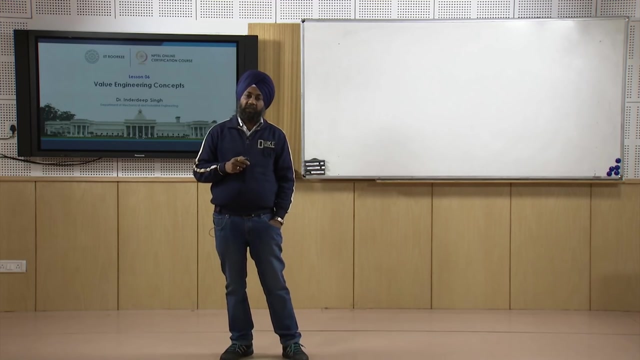 outrightly successful. so we will see some of those, those case studies also. so let us first try to understand. in todays session we will just have an overview of the value engineering concepts. try to understand the basic philosophy of this technique and try to understand the concepts of value engineering and try to understand the concepts of the. 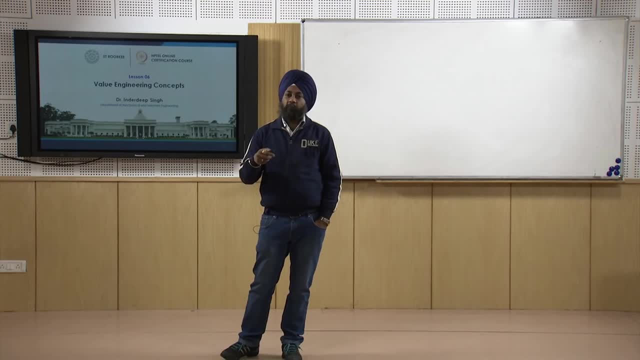 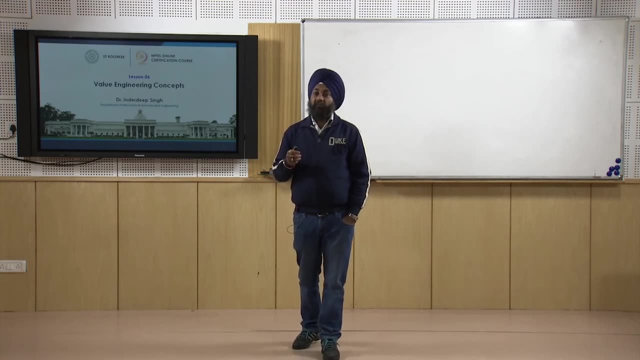 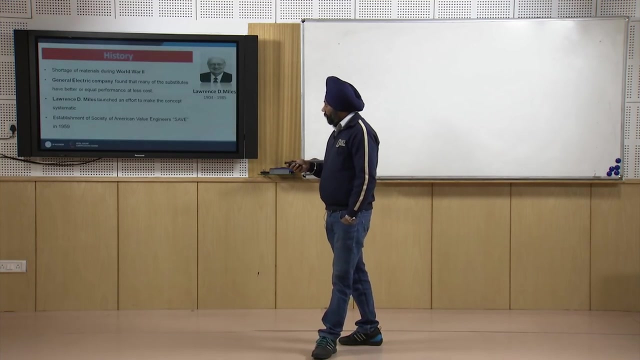 understand it with the help of some definitions and little bit of, we can say, historical aspects of value engineering, and we will also try to see that, what are the advantages that we can derive if we use the concepts of value engineering. so let us go, ah, one by one. so 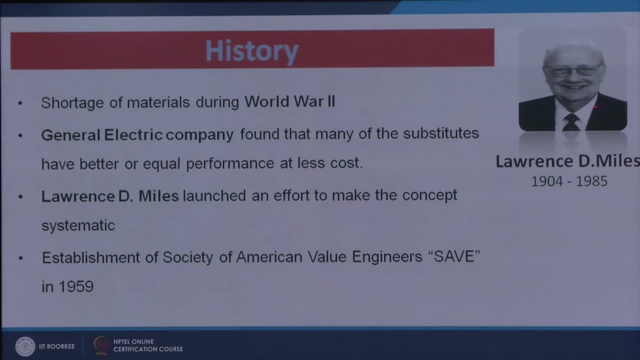 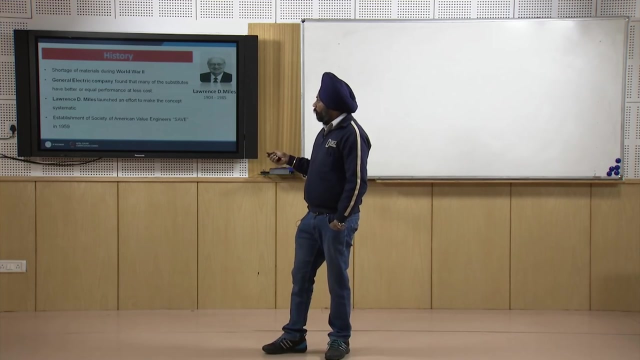 let us first see the history. this is lawrence d miles. he is considered as the you- we can say the pioneer figure or the leading figure in the field of value engineering and how the value engineering concept evolved. it evolved due to the shortage of materials during the 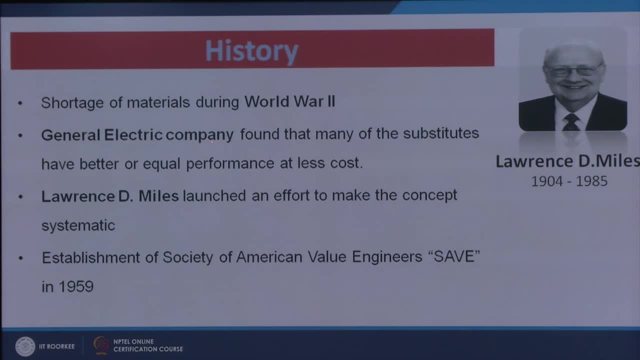 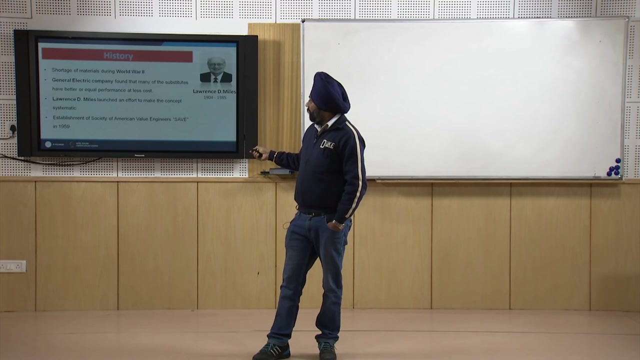 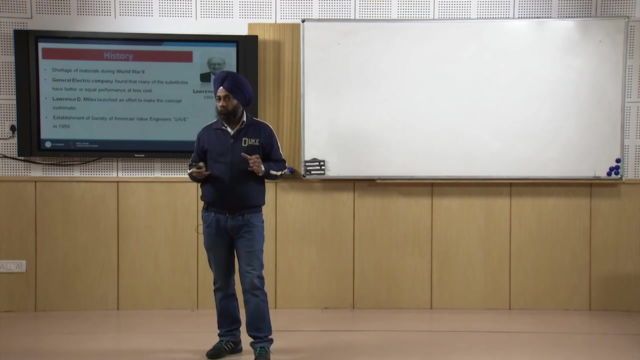 world war two and g e, that is, a general electrical company, found that many of the substitutes are better or equal performance at less cost. so, for any particular product, what do you need? you need the materials, materials or the substitutes. now it hap. it so happened that after the world war two or 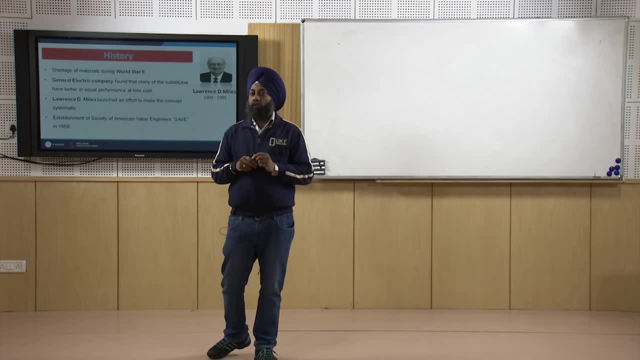 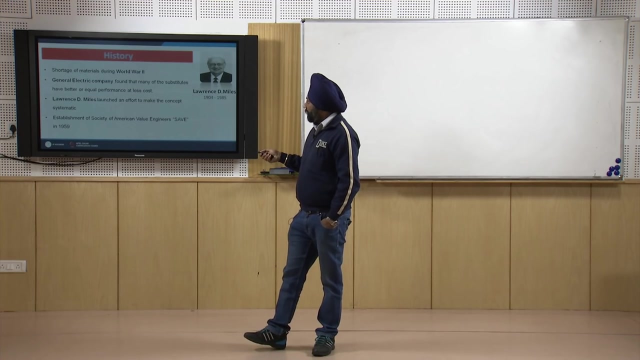 in some time, overlapping time. during the world war two, there was a shortage of materials shortage. the designs of a particular, we can say- artillery gun or a defense equipment were not available. so what did the engineers do? particularly, may be at journal electric, this concept was developed that why not to use alternate materials? 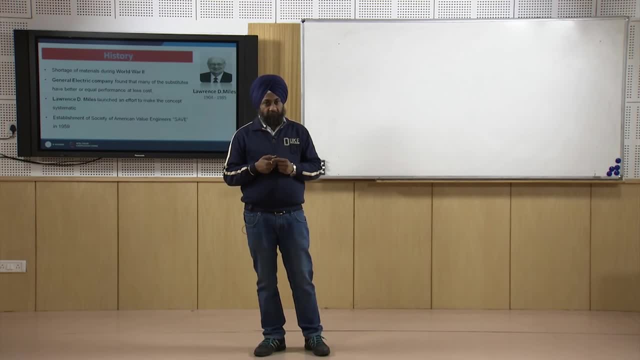 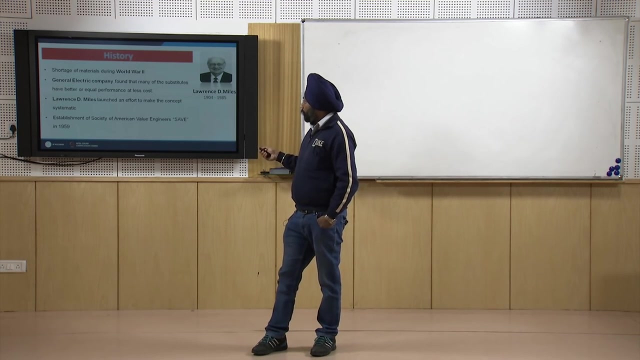 why not a, why not a, why not to modify the design, why not to change the process? so three common things, or three important things. i have said. material first is design process and the materials, or other order, design, materials and the process. so these three things, if you change, these are the substitutes. so 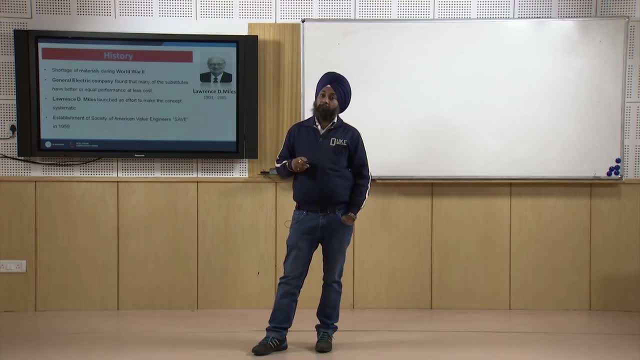 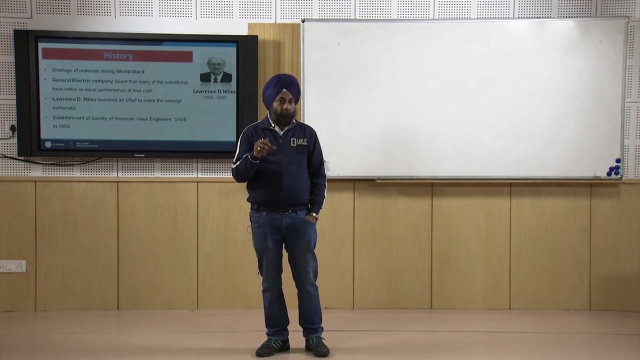 these led to better results, so substitutes were better as compared to the original design, original materials and original processes. so from there the concept evolved that there is always a scope of changing the product in context of its design material or the process used to make that product, and this is helpful for saving of costs. so the this was the basic. 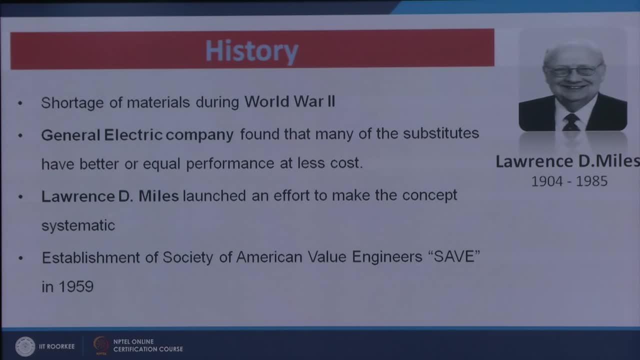 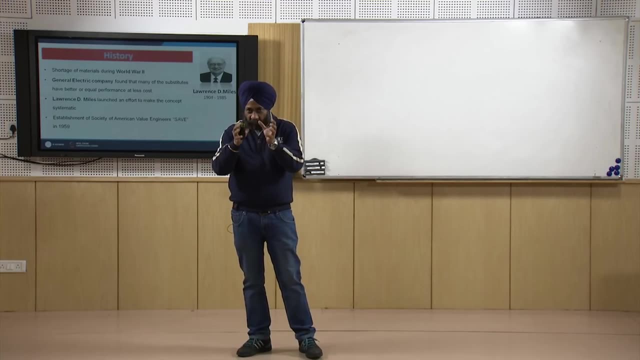 you can say triggering point of launching the concept of value engineering. then lawrence d miles launched an effort to make the concept systematic earlier. earlier it was not we can say systematic. the concept was more of philosophical thinking that if you change these things, money will be saved. 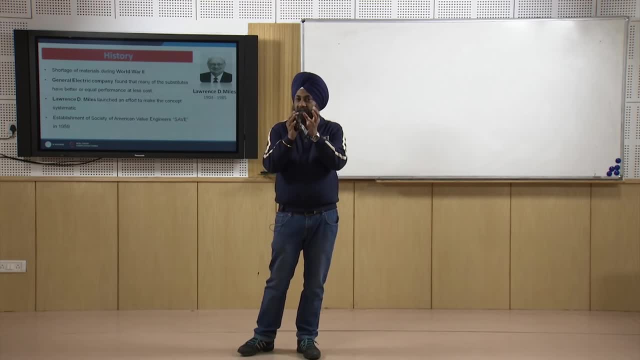 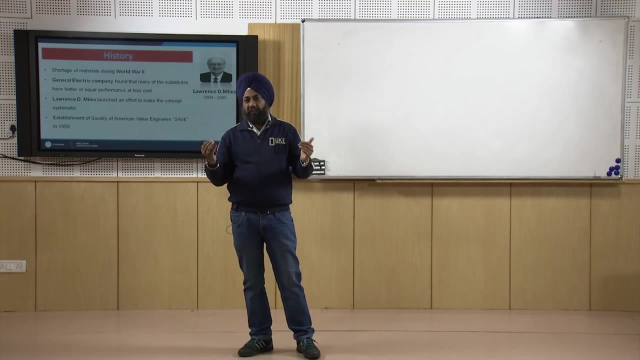 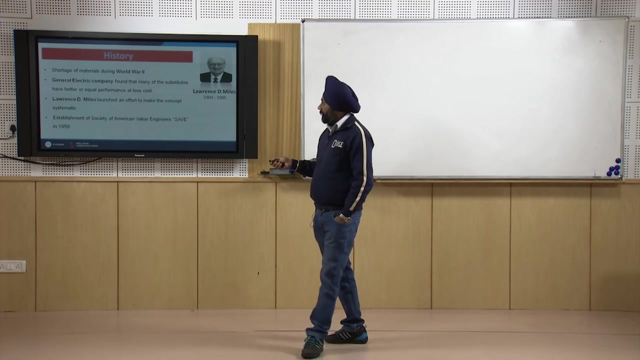 but then lawrence d miles took it as a challenge and then he tried to systematize, or put it into a systematic process, step by step process, so that anybody, any engineer, can apply these concepts and save the money for his or her organization. so this is the concept. 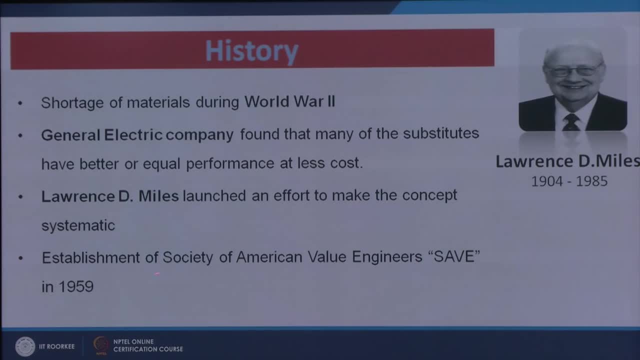 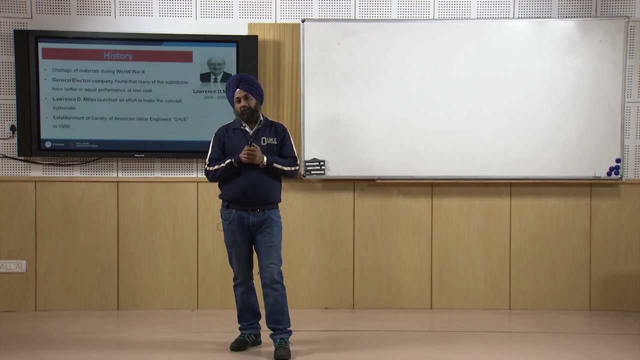 finalized by lawrence d miles, and this then it led to the establishment of society of american value engineers, save in nineteen, fifty, nine, to the all the concepts were then, we can say, put together and a society was, ah, established for propagating this concept among engineers and scientists. so this is the 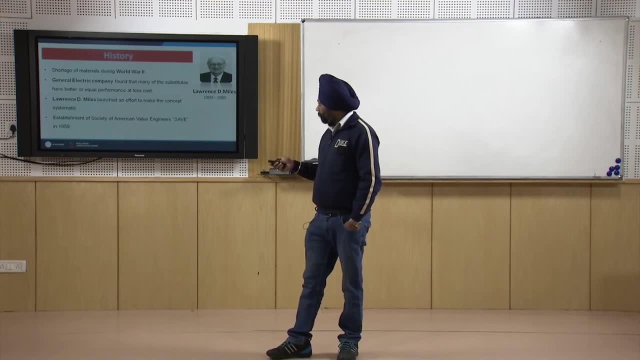 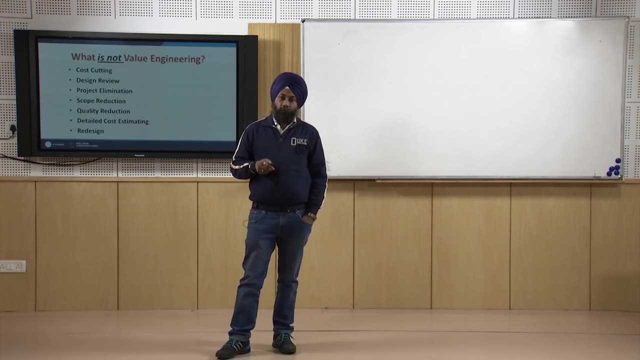 brief history of value engineering. now, whenever you have a new term on your platter, you start thinking that this may be similar to this thing, or how it is different from this thing, or how it is different from what we already know. for example, suppose we go and buy onions. 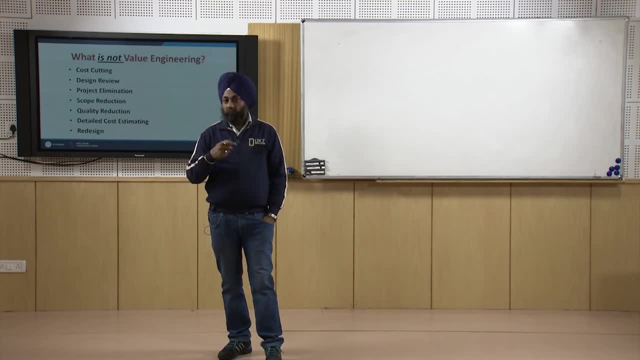 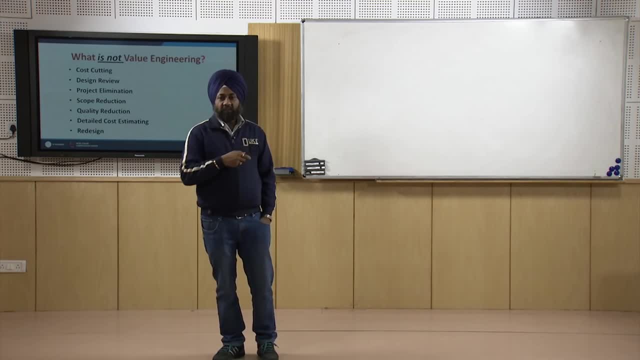 to the market. sometimes we go to three or four vendors, ask for the prices and wherever we get the minimum price, we buy. the quantity that we want to buy isnt it? i think all of us do the same thing now. it means we are doing value engineering. we have some target in our 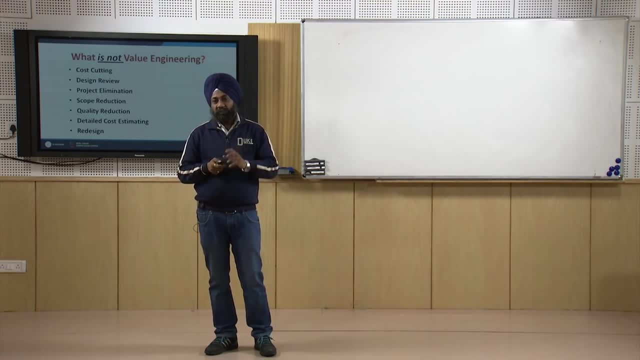 mind that what type of onions we want. what is the size of the onion? general quantity. what is the area, the strips of the leaf, regret 조. general quantity éof the divider, the whole process. does that not have any value to do with the value change process? think of aslah. 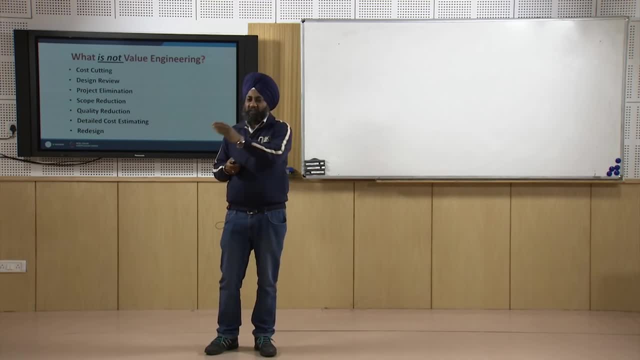 is awesome. side by side we- we generally jumps on the subject, we that go manage what we need. eastern bahce we. or what is the limit of the market? you can apply the average quantity, so it which is ideas, quality of the onions that we want to buy, and then we see three alternatives wherever 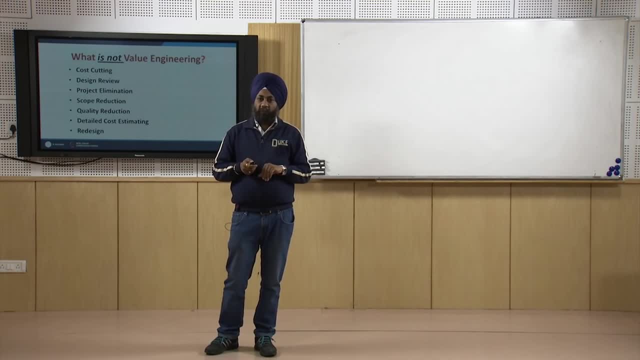 we are getting the cheapest alternative, we are buying the onions from that vendor. so, ah, everybody is doing value engineering, is he in his or her life? but the systematic analysis, if we want to apply the same concept in any engineering solution, for example this camera which is recording this lecture, if we want to analyze this concept or analyze this particular 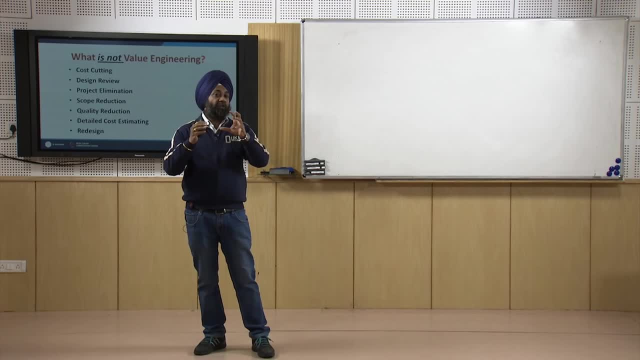 camera from the value engineering point of view. what do we need to do? it is not as easy as buying onions. we need to systematically break down the various components into ah individual component, then see what is the function of each and every component. then we have to see that can we combine? 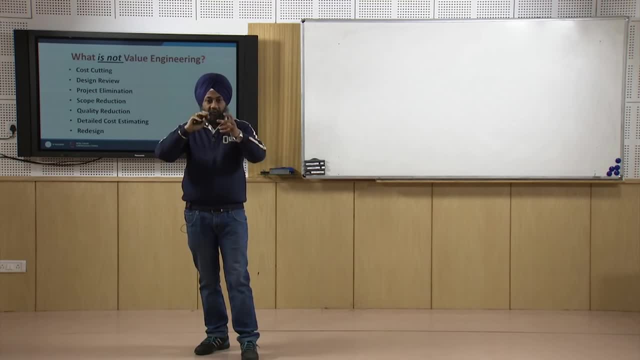 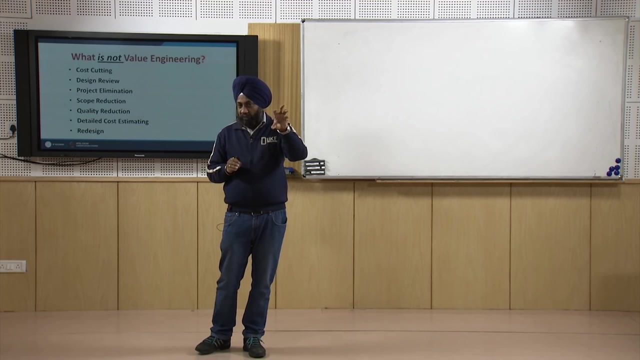 I mean some functions. can we eliminate some function? can we do some design modifications, keeping the performance same? the performance should not deteriorate or performance should not die down. that is our basic concept. so buying onions for same quality or same taste or same package or same look usually. 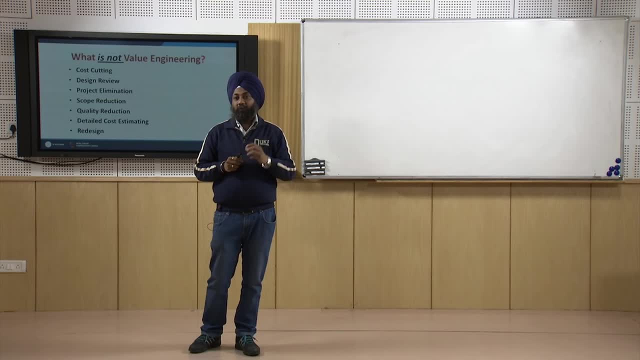 by taking into account it should be good looking, also not good looking as a person, but it should should have a good packaging. it should not be stale, it should not be. you can say poor quality, so our quality is same. we are comparing three alternatives and whatever quality standard, 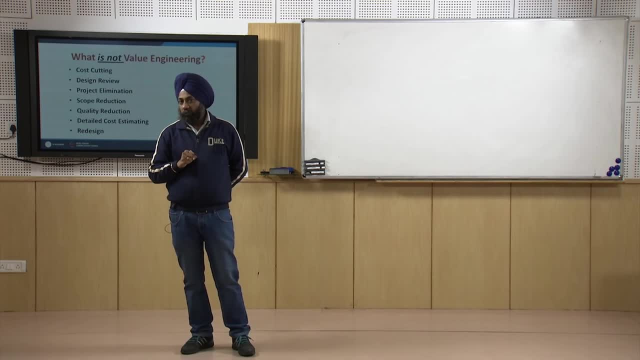 we have set. we are picking it up similarly for the camera design also. we need to keep the performance standard same. no change in the performance standard, but we have to redesign it in such a way so that, the performance remaining same, the cost comes down. so that is the basic. 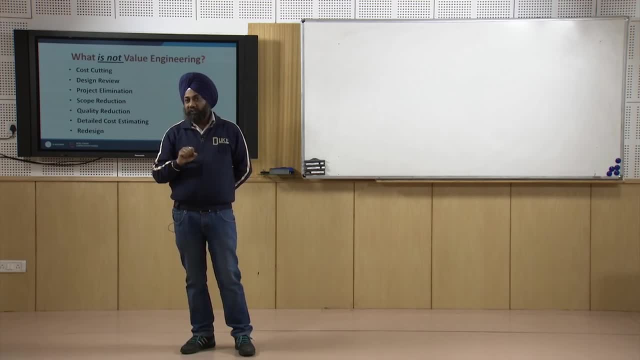 the basic concept of value engineering. so everybody is doing value engineering is in his or her life, but a systematic way of applying the these concepts we are going to focus during this session. so let us quickly ah see what is not value engineering. so value engineering. 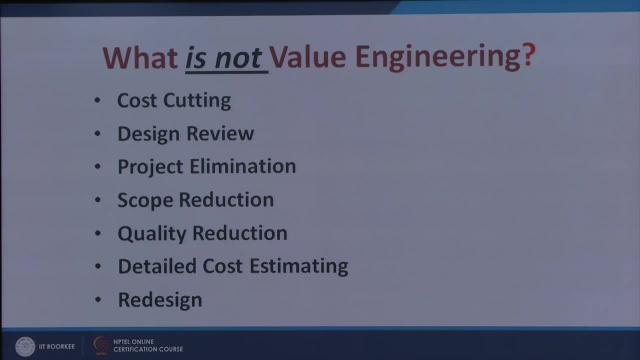 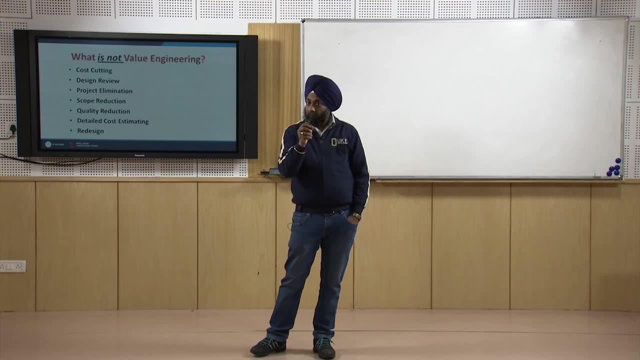 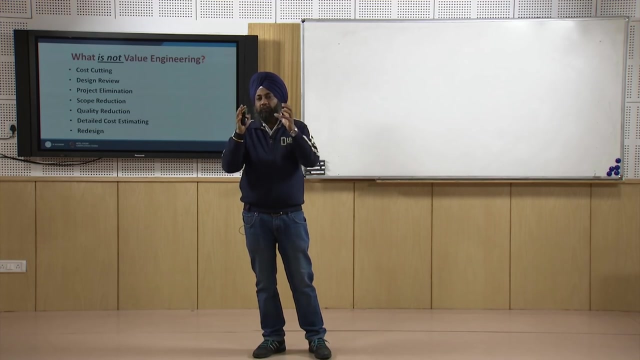 is not cost cutting. many people say when you are saving money it is cost cutting. no, it is entirely different. the focus area is entirely different. must i tell you that in many cases the cost will increase. in many cases, when you apply the concept of value engineering, the cost may increase but the overall cost of that particular project would reduce may. 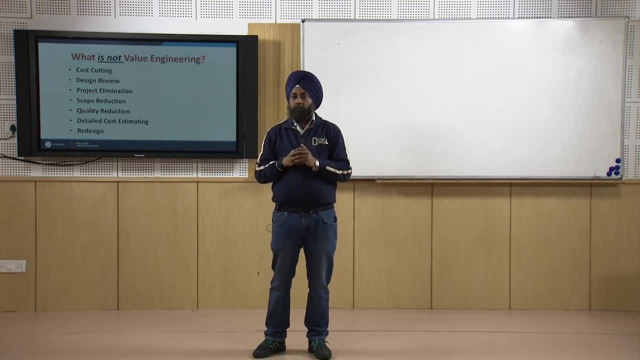 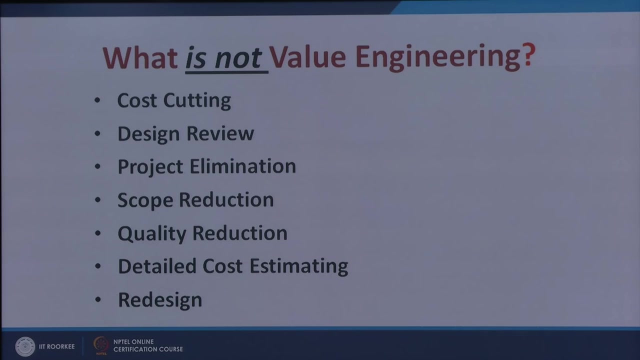 be when considering the life cycle cost of the project or the product. so it is not cost cutting. in many cases the cost may further escalate on applying value engineering, but the overall value of the product would certainly increase. so it is different from cost cutting. we will see in one of the subsequent lectures that how exactly it is different from cost. 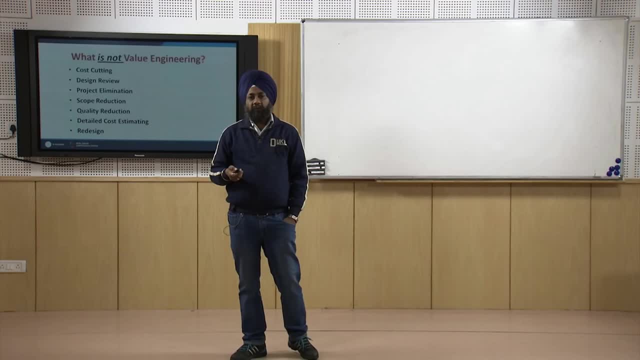 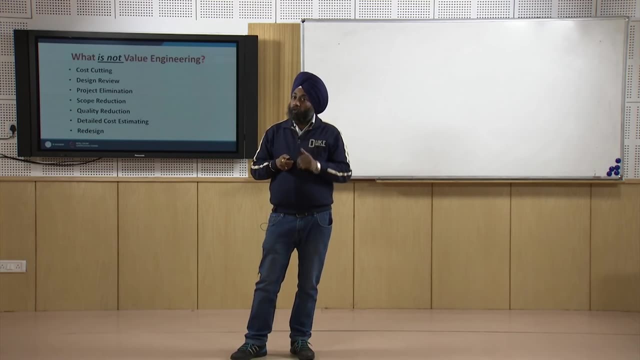 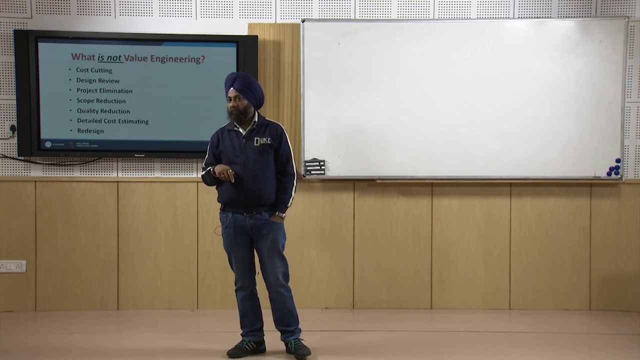 cutting. it is not designed review. some of the people may say there is a design, then few- few you can say persons will evaluate that designs based on the cost. no, it is not designed review, it is a design process itself. in this we will see the concepts of value. 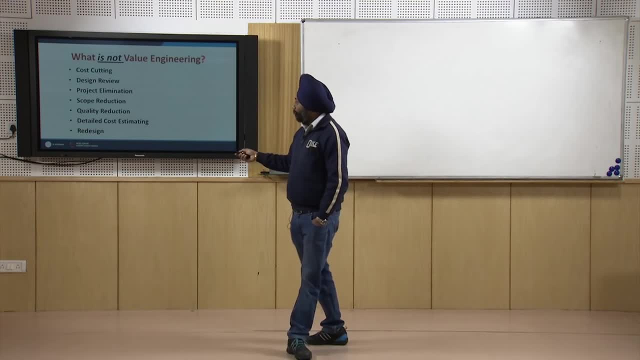 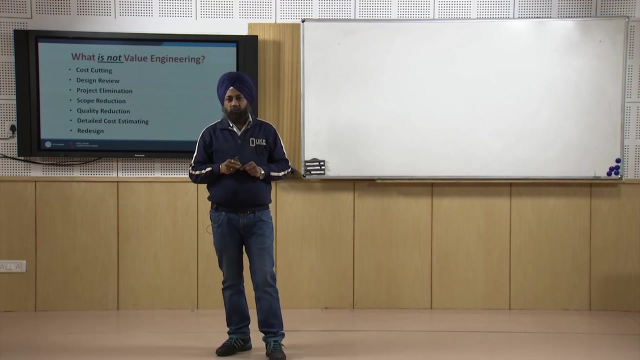 engineering and we will design the product as per the value engineering guidelines. so there is no review or this is not a design review process from cost point of view. it is not project elimination that if you have may be three or four different ah projects available, so you will see which one is cheaper, so select the cheapest project. no, it is that. 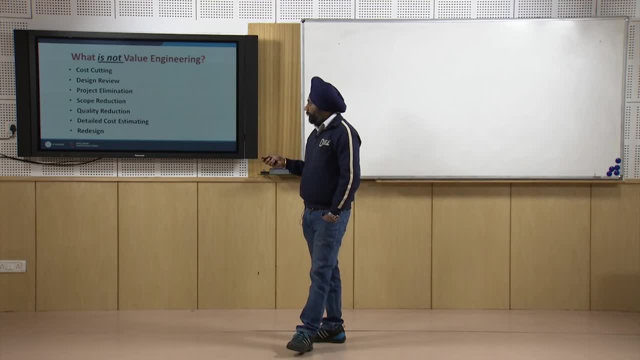 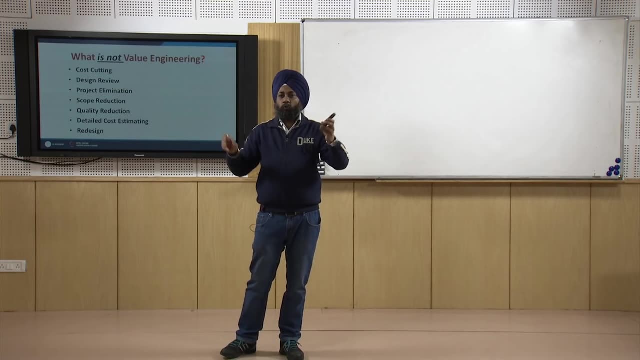 is not project elimination, it is not scope reduction. sometimes people will say that for this camera, if you apply value engineering, it may eliminate one or two parts, so the overall scope of this camera will die down. no, that way that is not the case almost, or i should say, even there can. 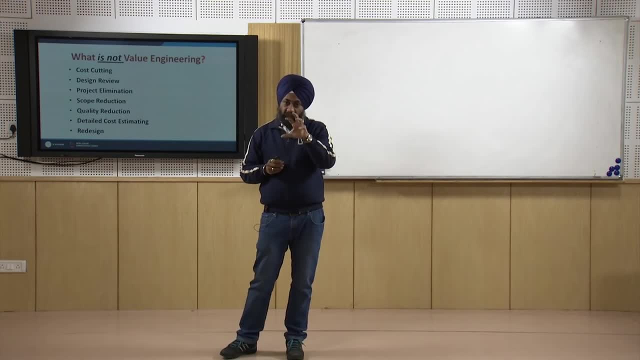 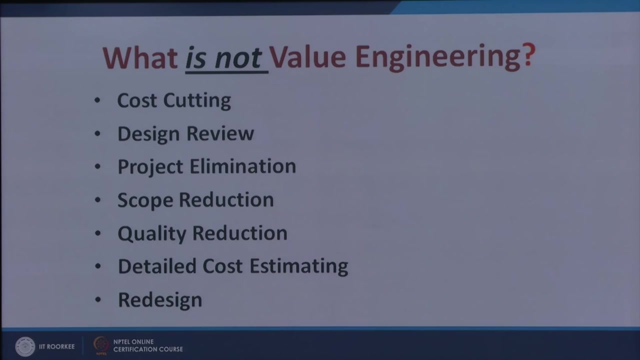 be increase in the functional value of the product after the value engineering process. so it will never lead to scope reduction, but i can say with confidence that the scope may further improve. that is one advantage of value engineering: quality reduction i think i have today only within last seven to ten minutes i have told, i think, three times that there. 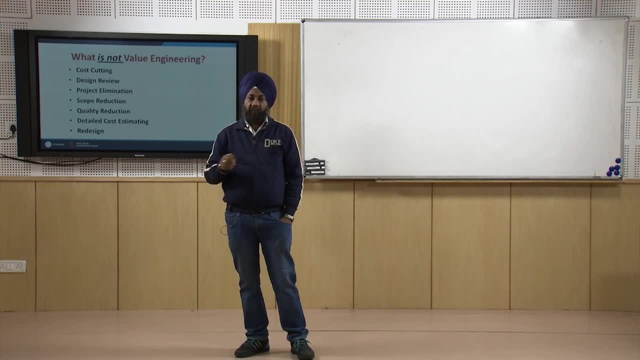 has to be no compromise on the quality, performance, reliability, serviceability. no compromise anywhere. only thing is using the fundamental aspects of science and engineering and using a common sense. we will aim to bring the cost of the product down by our, our creativity, innovation, as well as the knowledge that the engineers gather over a period of time. so there will be no compromise on anything that is quality reduction as well as the quality reduction skills as well. that is the key importance of value engineering. we will discuss the next one. i will discuss the next one after a long break, except for the next issue. so i will meet you again next week for the next issue of the technology and industry, any more. 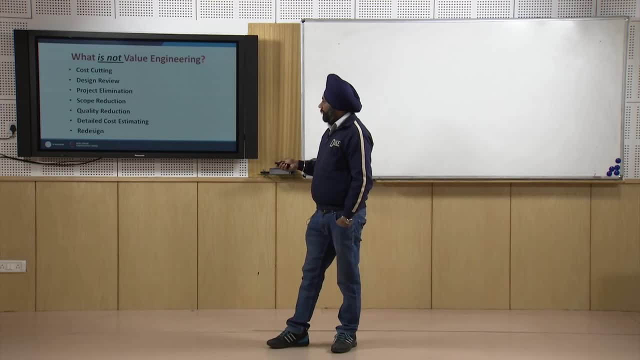 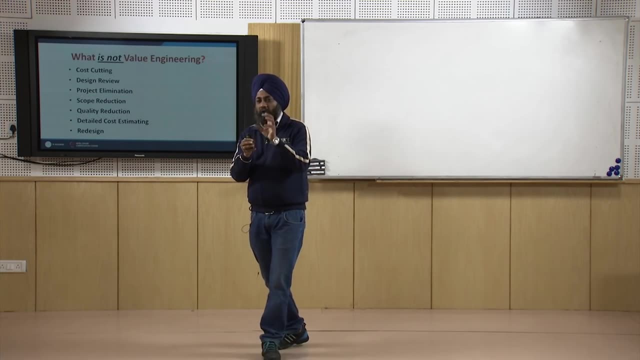 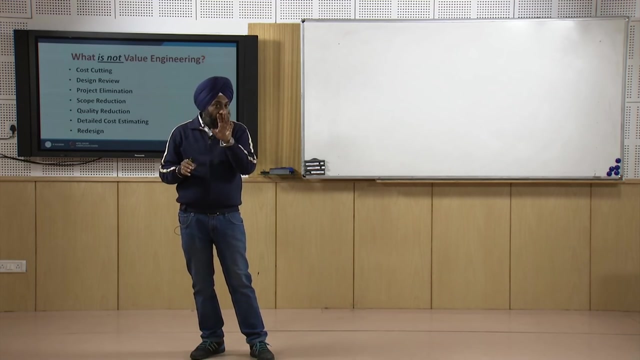 reduction is not value engineering. detailed cost estimation is also not value engineering. and redesign: you can say slightly, maybe in value engineering we may suggest some new designs, but it is not only the redesign process, only redesign process. maybe you design the product without considering the cost aspect. no, in this case, if even if we are redesigning, 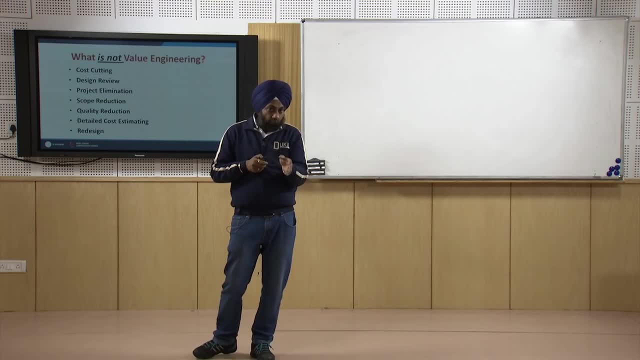 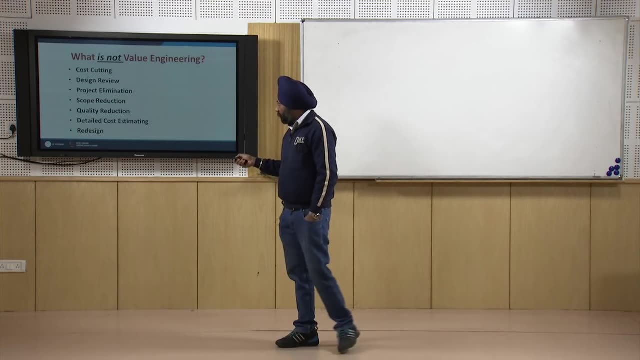 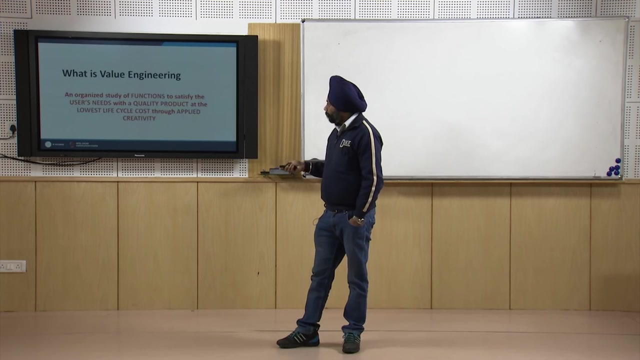 we will take into account the cost aspect also. therefore, value engineering is not the redesign process. it is entirely different process. so we can see: this is this, is this? the? all these points have nothing to do with value engineering. value engineering is a different aspect. now some of you may be wondering: what is a value engineering? why question mark is? 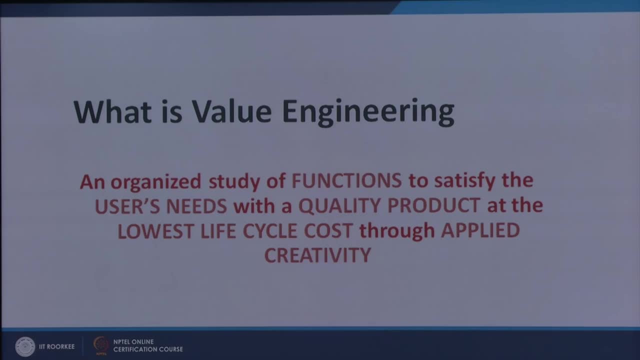 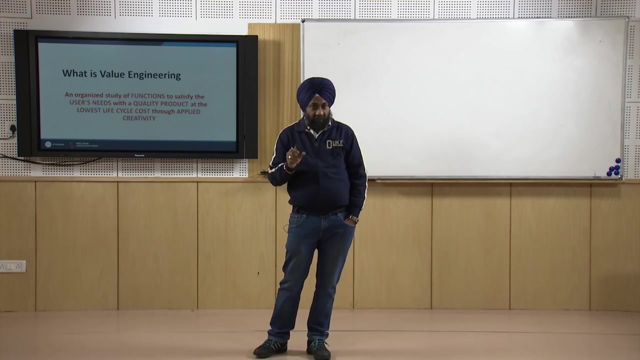 not put here because the answer is given. maybe on the same slide. you can see what is value engineering: an organized study. so let me first emphasize on an organized study. so it is not philosophy, it is organized, it is systematic, it is step by step, so it is orderly, so it has a sequence. 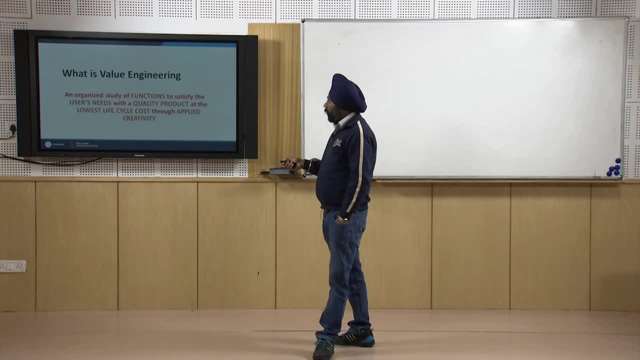 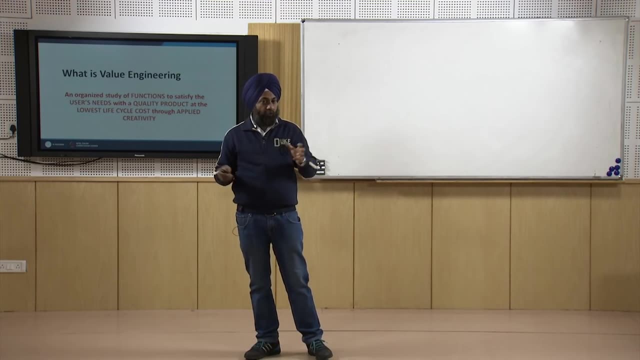 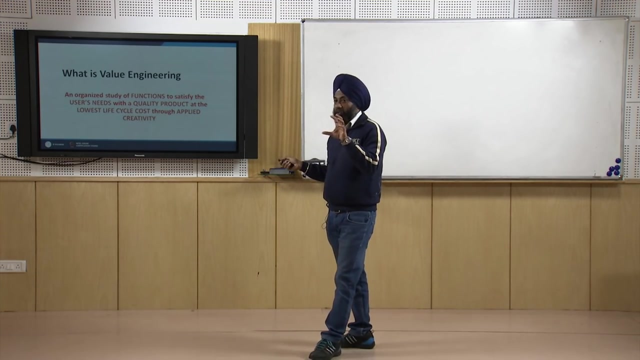 so it is a systematic or scientific study, so an organized study of functions. i have already told, with the help of example, that each and every product that the customer buys has a function, so you have to take into account that function. so it is organized study of the functions to satisfy the users need. 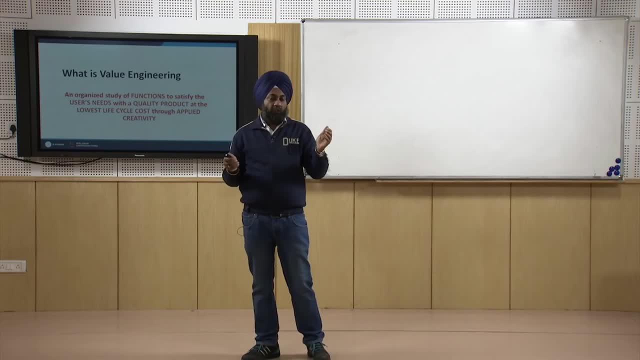 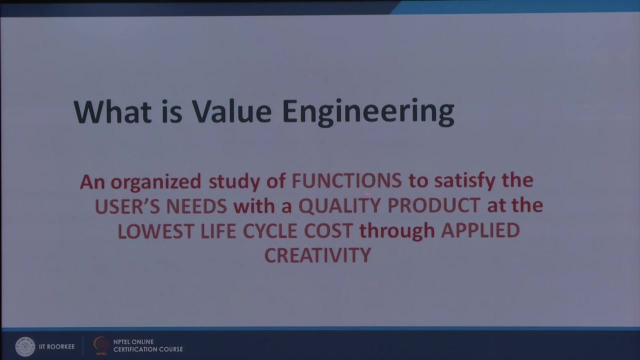 that we have seen why do we design products. in the last week we have seen that products are designed to satisfy the fulfilled or the unfulfilled or the new needs of the customers. so the functions: it is focusing on functions to satisfy the users need with the quality. 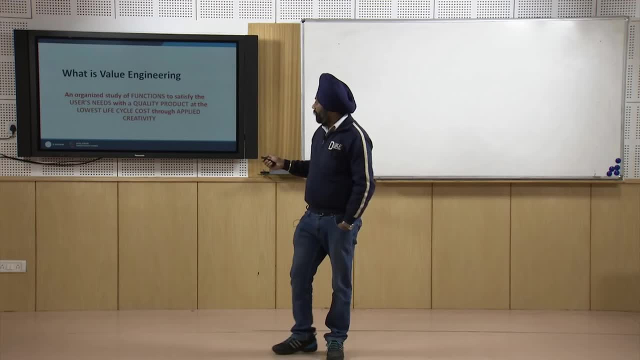 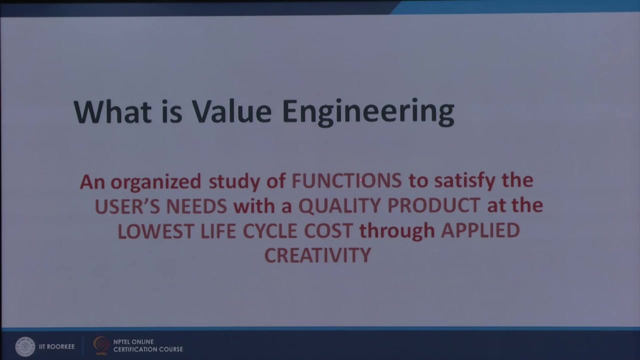 product. so quality cannot be compromised in this at the lowest life cycle cost through applied creativity. so let us see one by one: there is a user need for some functions which have to be satisfied, ensuring the quality at the lowest life cycle cost, and how it is possible by applied creativity. so you can see- i will not look at the ah explanation- 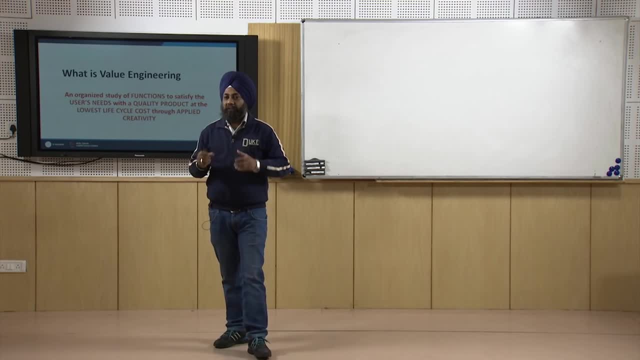 or the definition again. definition again. let me just try to clear this definition to you, because the next two definitions i am just going to read and move forward with our discussion. basic definition out of this definition can be that we have to achieve the desired function. now why desired? 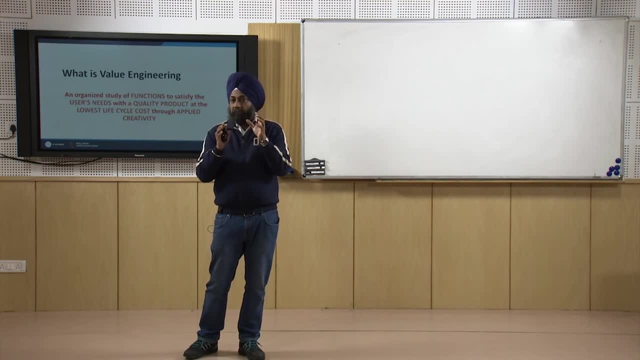 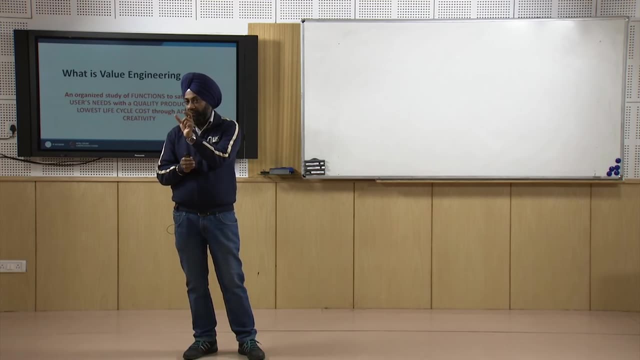 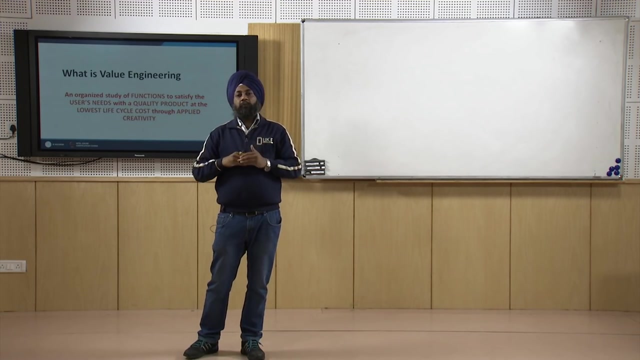 because the user wants that function to be achieved. so it is the process of ensuring, or it is to achieve the desired function reliably at the minimum possible cost- reliably is a quality parameter- or we can say it is to achieve the desired function at the defined level of quality but at the minimum possible cost. 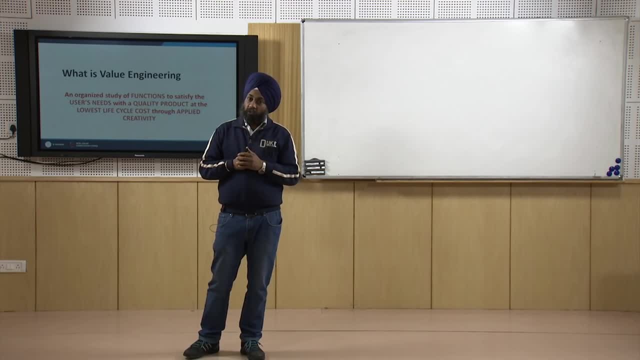 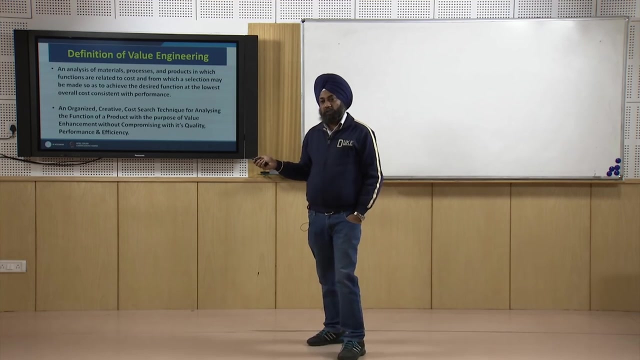 so that is what value engineering has to ensure. so again, it is emphasized that there has to be no compromise all in the quality as well as the performance parameters. so let us now see the other definitions. i will read these definitions for you. value engineering is an analysis of materials processes. 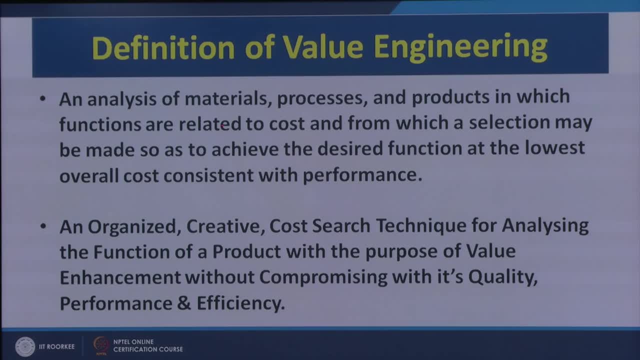 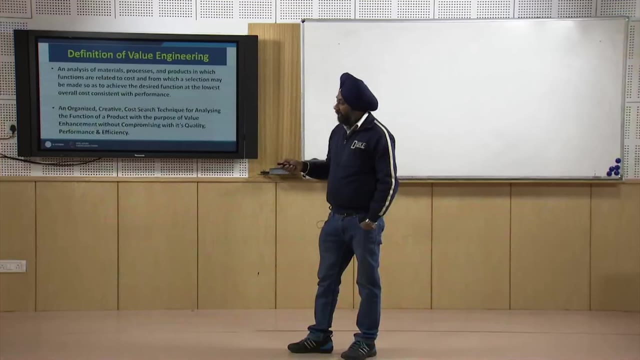 and products in which functions are related to cost, as i have already told, and from which a selection may be made so as to achieve the desired function at the lowest overall cost, consistent with the performance. again i am reading: to achieve the desired function at the lowest overall cost, consistent with the performance. let us see the second definition. 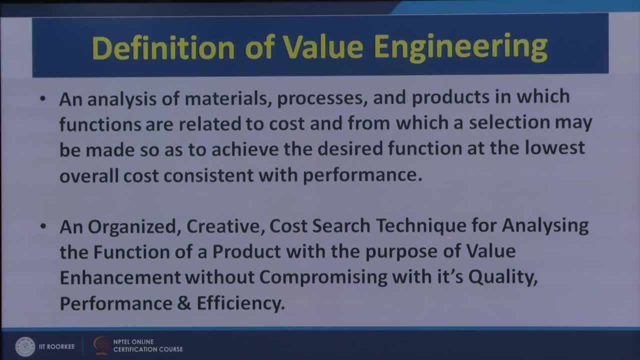 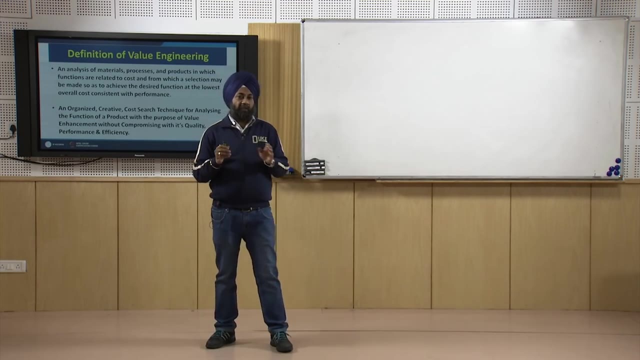 it is an organized, creative cost search technique for analyzing the function of a product with the purpose of value enhancement, without compromising with its quality, performance and efficiency. so i think the concept of value engineering is now absolutely clear to everybody: that it is to ensure that desired function is achieved. 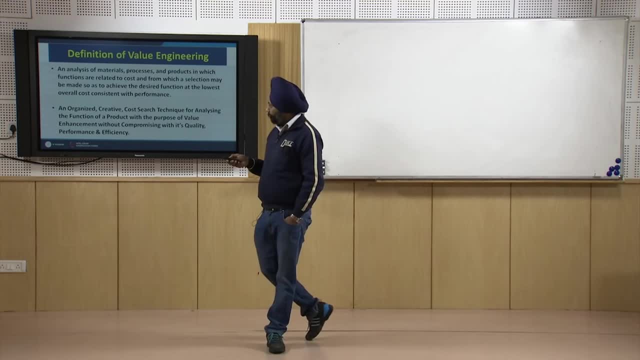 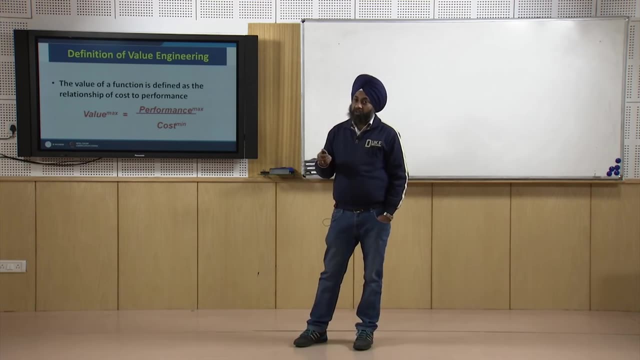 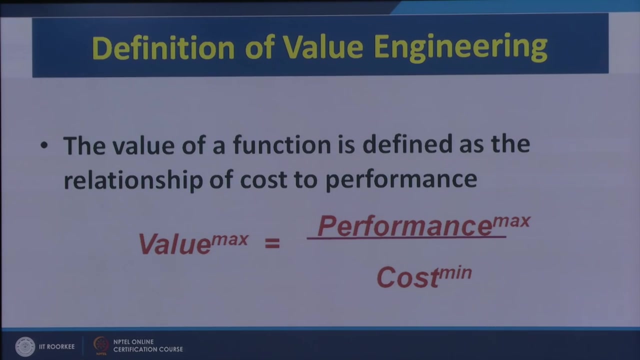 reliably at minimum possible cost. now if you see mathematically how you can relate this relationship, or how you can put this into mathematics, the value of the function is defined as the relationship of the cost to performance. now, v max is equal to performance maximum divided by cost minimum. let me emphasize here in place of performance. in many books or in 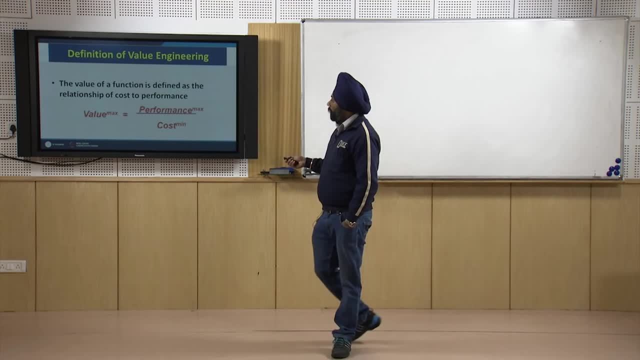 different types of literature, you will get function also. so it may be written as: value is equal to function by cost. so v is equal to f by c. so this, this is a relationship between three things: value of the product, for example this pointer can have, can be considered as: 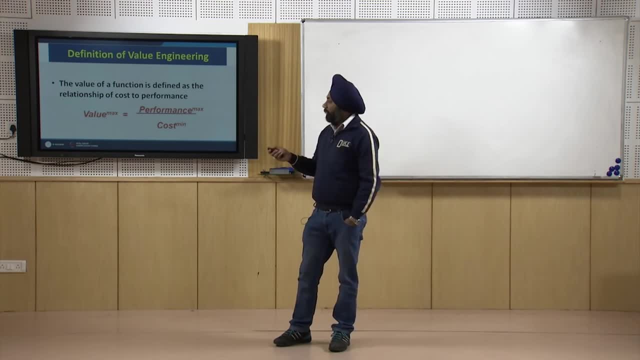 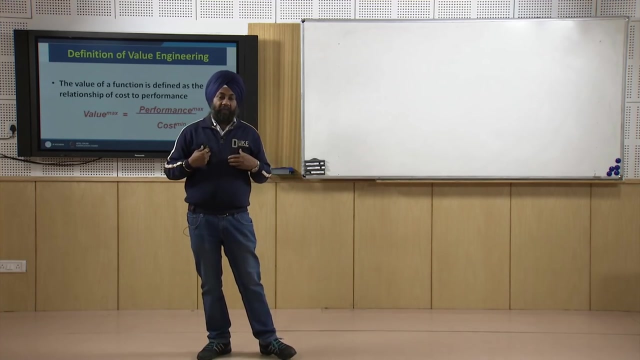 a product, all right. or the jacket can be considered as a product, so value of the product is directly proportional to its performance or the functional value of that product and inversely proportional to cost. so very easily i can say that this jacket can have a very good value if it pro provides me the warmth for which i have bought. 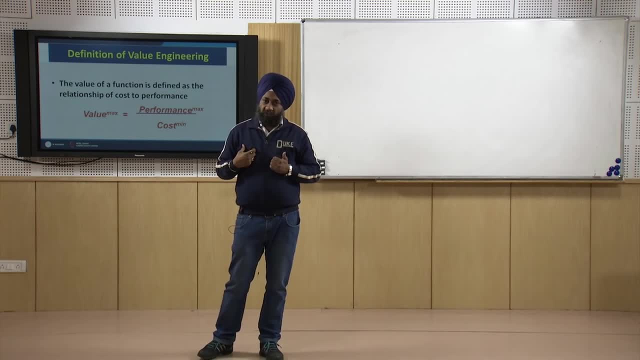 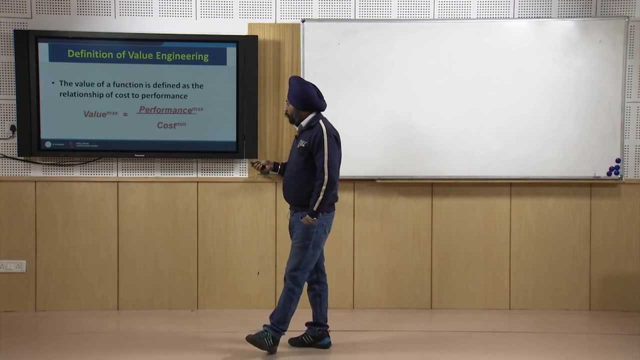 this jacket and i have to pay less money for the buying this jacket or for acquiring this commodity or for acquiring this product. so it is directly proportional to the functional value, inversely proportional to the money that i have to spend to acquire that product. so value and as a value engineer, what should be my target? as a value engineer, my target 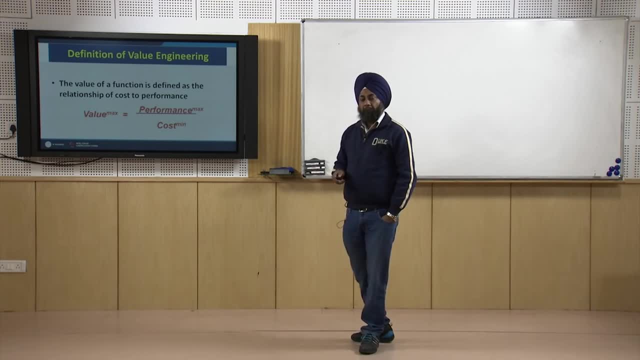 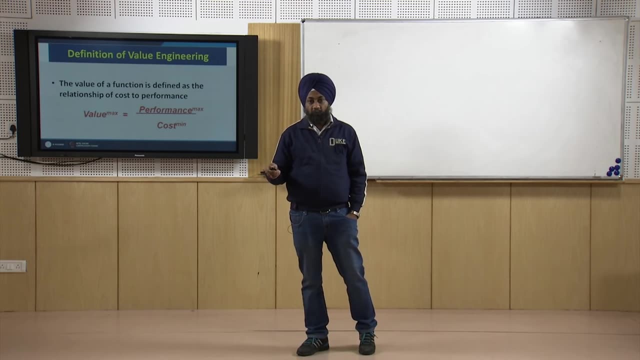 is to maximize this value, maximize and minimize the cost that the customer has to spend. how it is possible? providing the functional value, high functional value for that product. so this is the value of the product and, as a value engineer, what should be my target as a value? 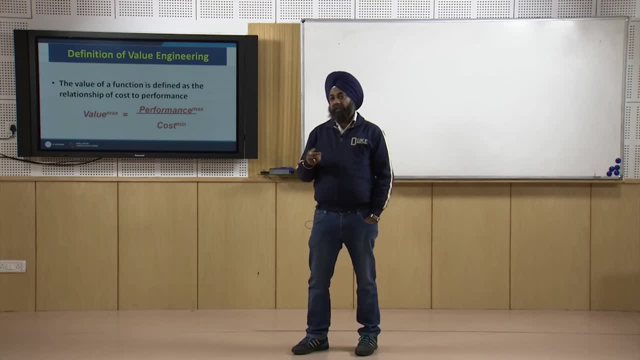 engineer is to maximize the cost that the customer has to spend. how it is possible providing the functional value acting as a value for that particular product in a very highly25? it requires a lot of search, it requires lot of innovation, it requires lot of creative thinking. they are only there after only you will be able to come up with ideas which will 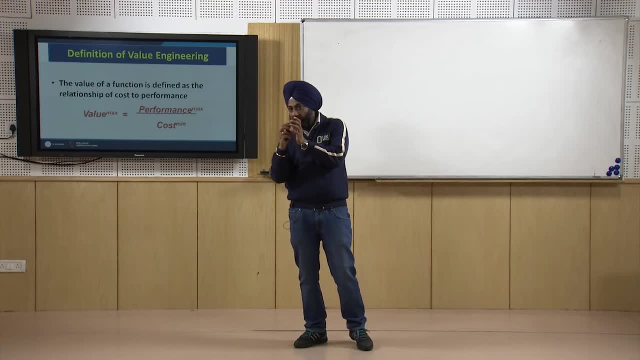 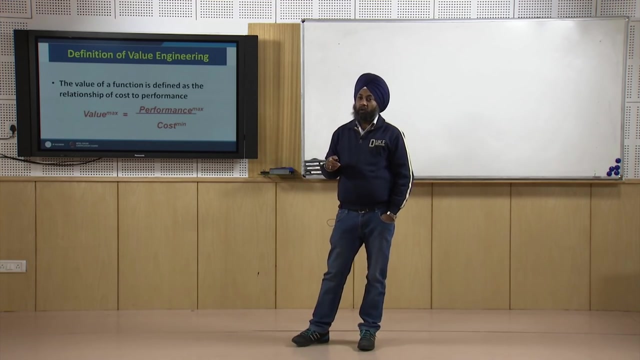 help you to redesign the product or which will help you to select a alternate material for that product or which may help you to suggest uh alternate manufacturing process for that product so that your cost is minimized. wi basic concept of value engineering and how it can be related mathematically. how value 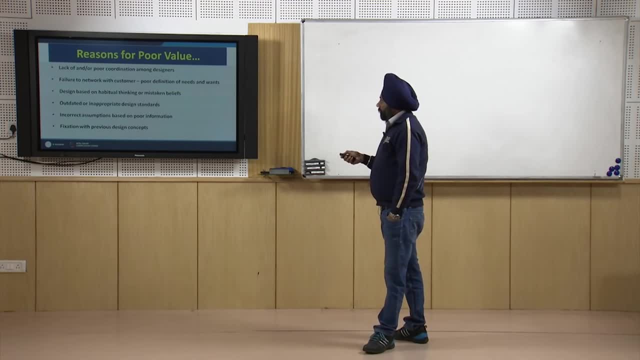 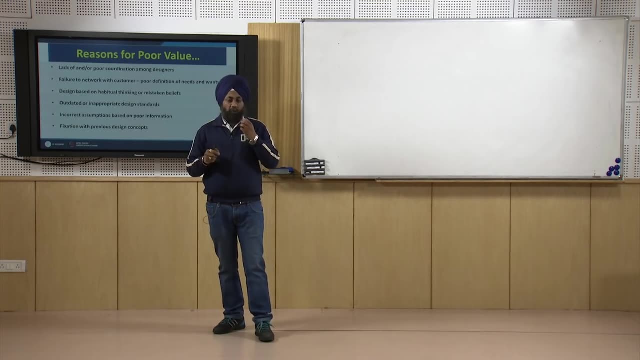 can be related mathematically. so some of you may be wondering now if i think you have understood the basic concept of value engineering. some of you may be wondering that i am using a jacket, how it can have poor value, or why do we need to do value engineering so prior to. 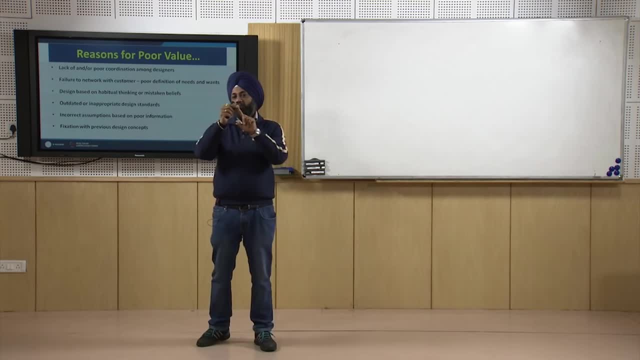 that i may emphasize on three words. first one is value engineering. in number of books you will find value analysis and value management, which is not a very common term. but value engineering and value analysis are used interchangeably and people are usually not able to understand the difference between the two. so value engineering are the concepts when they are applied at. 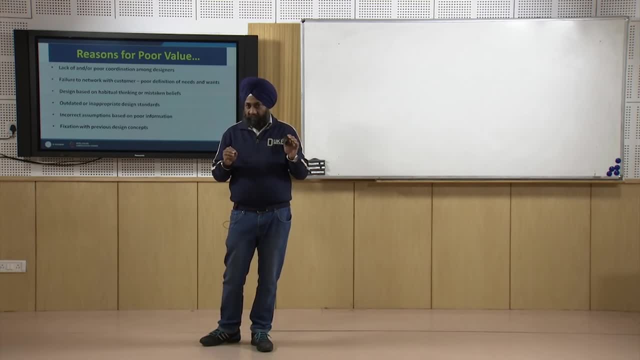 the product design stage. design stage means i have a idea that i have to manufacture, maybe a pointer which should be able to have dual functions, that is, it should be able to point on at the screen and it should be able to change the slides also. now, if i apply all my value engineering concepts, 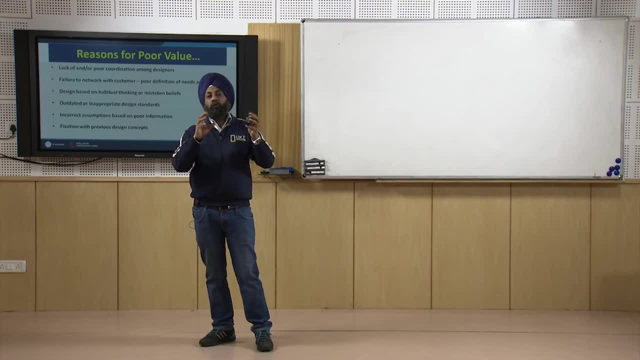 and during the design stage of this pointer, i am doing value engineering for this product. now, suppose this is already in my hand. it means the product is already existing and i am using it or the other users are using it. now suppose i want to apply the concepts of value engineering on this. then i will see. 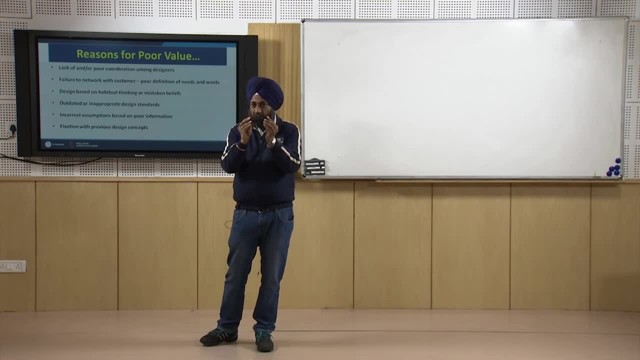 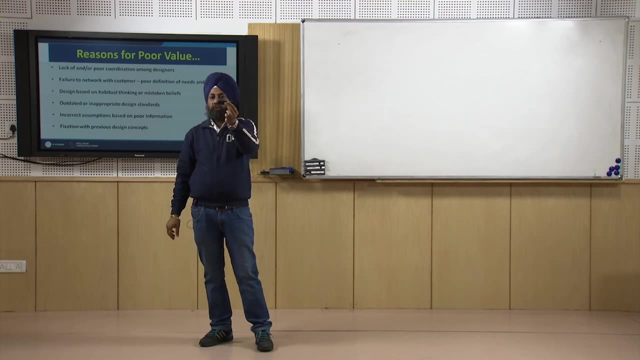 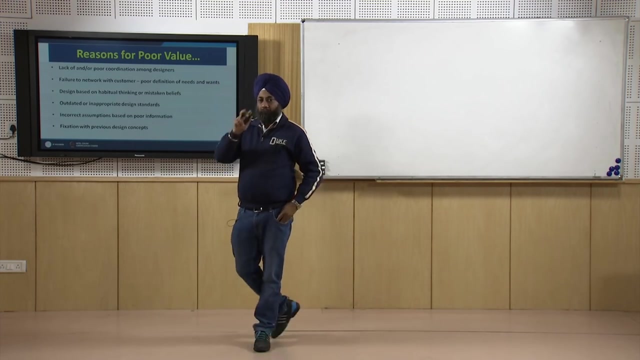 what are the desired function and how i can achieve both the functions reliably without compromising on the performance, but at a lesser cost, then i have bought this product, all right. so then it becomes value analysis. the product is already there, the functions are already being achieved, but i further want to analyze it from the cost point of view. ok, 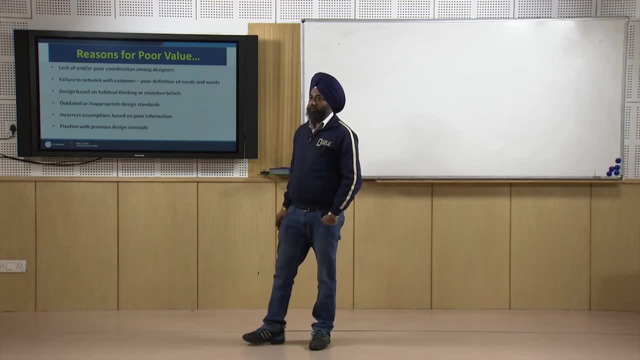 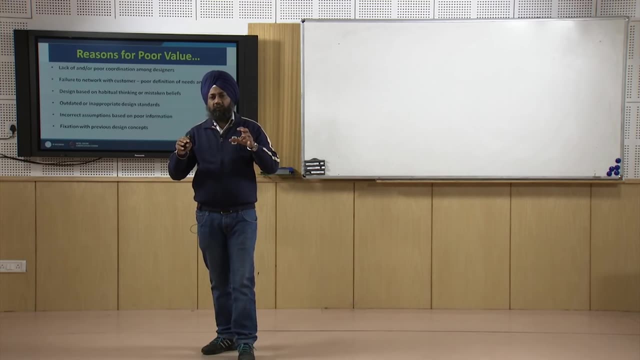 so that is the point: basic concept of value engineering and value analysis. now these points list out that why these products? why do i i analyze, why do i want to analyze this product? for value or on. in other words, we can say: why should i do value analysis if already? 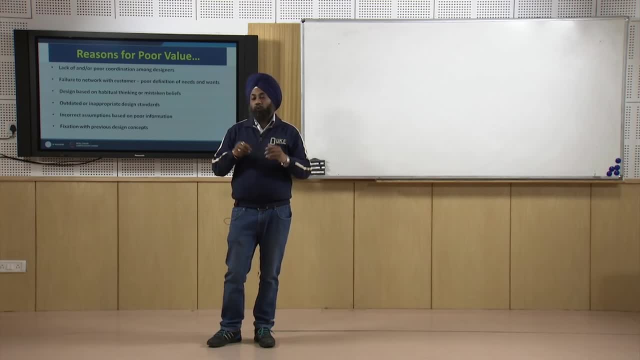 i have done value engineering during the design stage. ah, so these are the reasons that why products sometimes have poor value and therefore they need to be analyzed for further improving their competitiveness in the market. because, if you remember the product life cycle that we have covered in our last week, there is 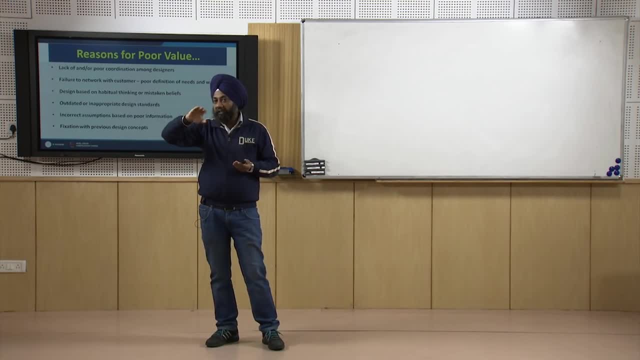 a maturity stage and at maturity stage the market share of the product is more or less constant. so the company may, would would like to become more competitive by offering discount to the customers, discount on the product to the customer. now how the company will give discount if they are able to save some money in the cost that is adding up to make that. product. so at that point of time companies may want to do value analysis of the product so that they use now alternate materials or manufacture it through alternate process, or they can redesign it slightly so that the overall cost of the product comes down and they pass on the benefit and return to the product. it would be less cielo return to the 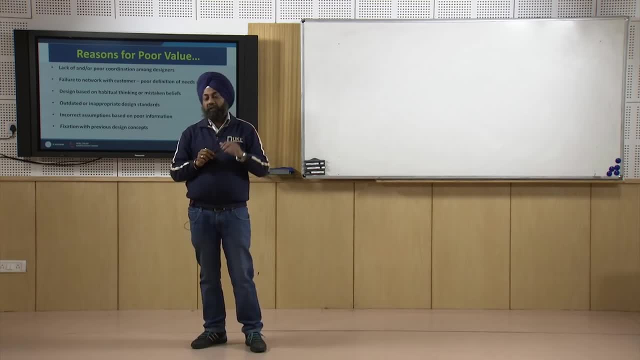 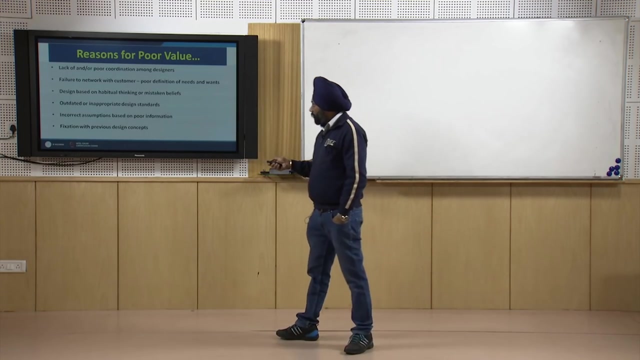 benefits to the customer and try to get more market share during that maturity stage. so therefore, the value analysis is equally important as compared to value engineering, which is applied at the beginning or at the design stage of the process. now let us quickly read these parameters. what are the reasons for poor value in a product? 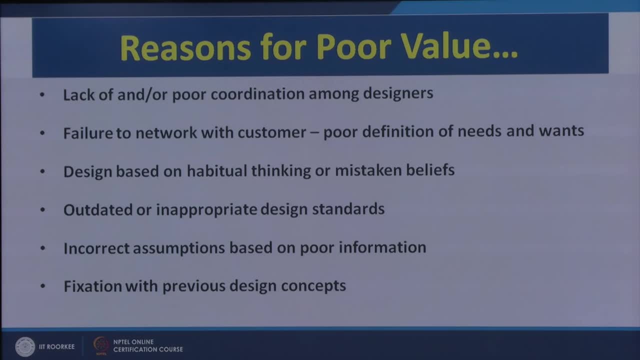 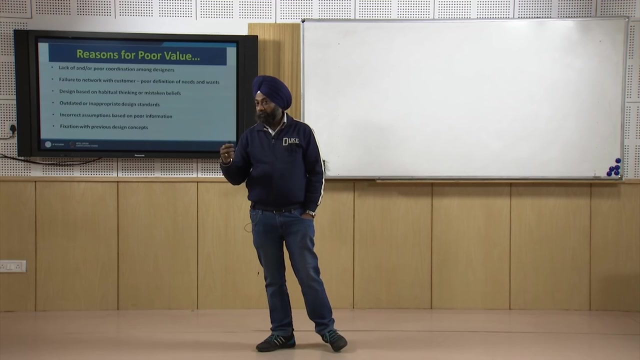 first is lack of or poor coordination among the designers evident. if designers are not in harmony, the product may have poor value. failure to network with customer, poor definition of needs and wants. we have not been able to find out the functions that the customer is desiring from the product. so our marketing or our marketing aspects have not been addressed. 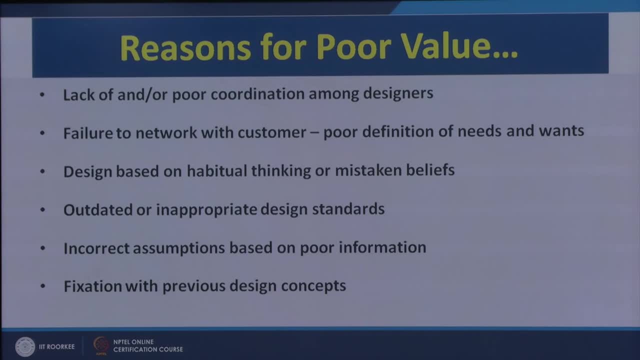 properly. design based on habitual thinking or mistaken beliefs usually change. people do not want so. whatever is the our design thinking we dont want to change, which leaves leads to poor value in the product, outdated or inappropriate design standards clearly evident. the company may be following the design standards for the last twenty years and many 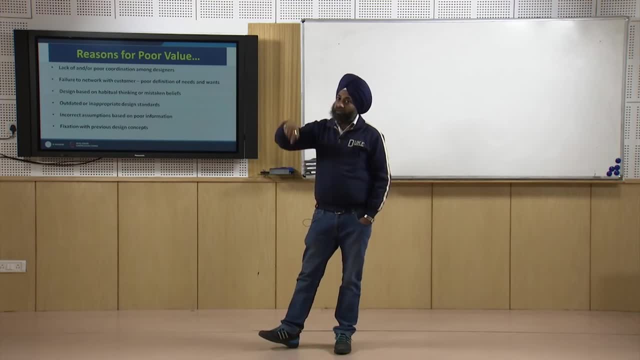 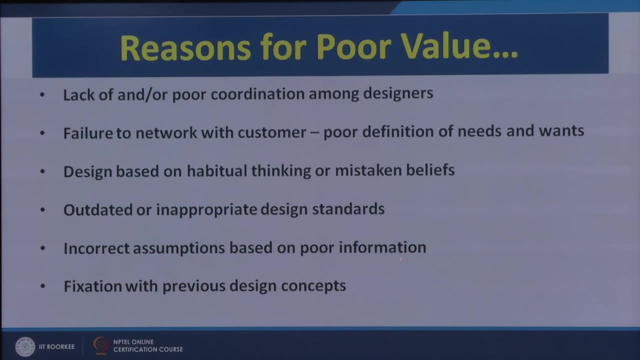 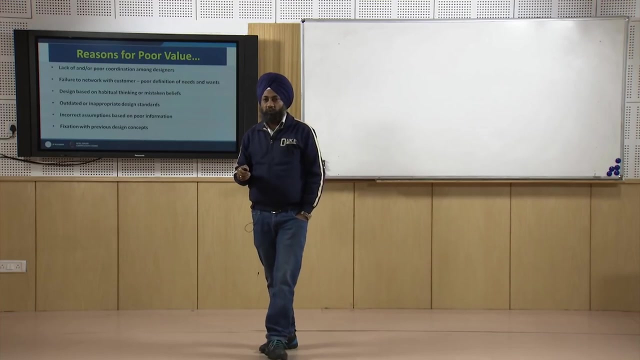 things may have changed over a period of time. therefore, if old things are used, you may not be able to launch a product which has good value. then incorrect assumptions based on poor information. so information is not adequate. fixation with previous design concept. so whatever tools and techniques were used by the earlier designers in the company, same things are continuing. 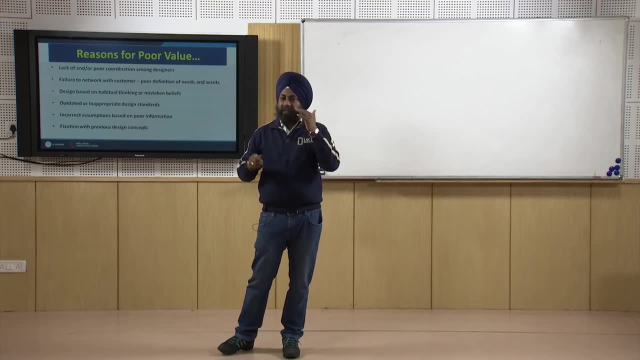 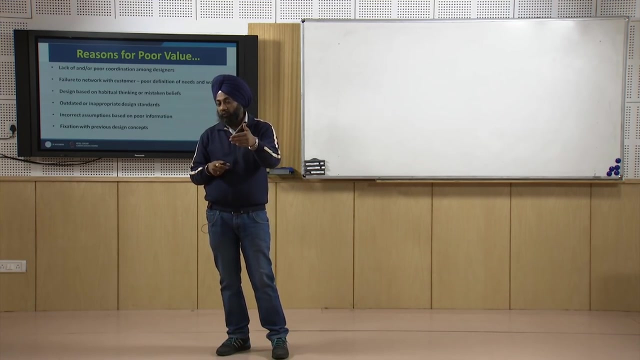 therefore, the poor value may creep in into the product. there can be other reasons also. a during our discussion, we will keep on identifying these reasons which lead to poor value and with case studies, we will see that: why this poor value has entered into the product and how, using the concept of value engineering, this poor value was eliminated, or the parameters. 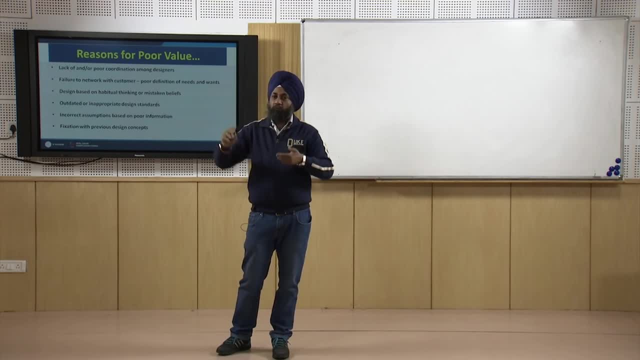 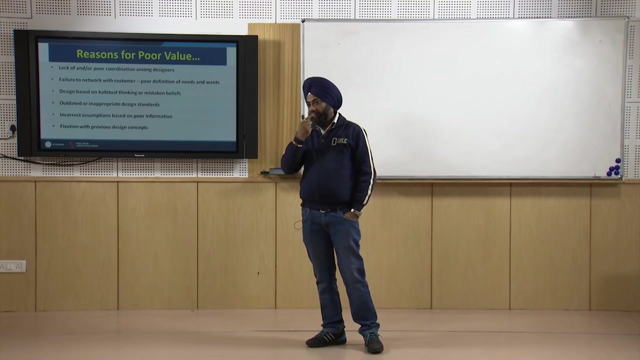 or the functions leading to this poor value were removed from the product and a product that was the redesign was better as compared to the previous product, which was not value engineered properly. so these are only ah some reasons which are responsible for poor value in the product. there are other reasons also, which 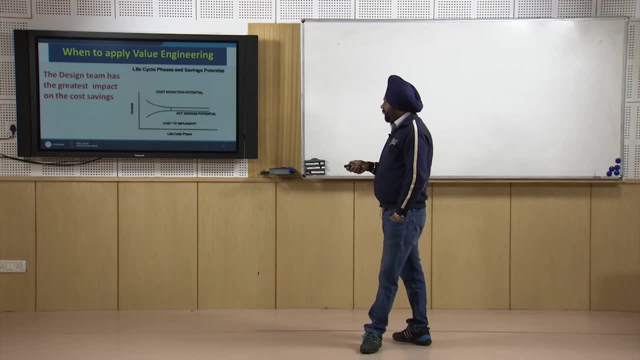 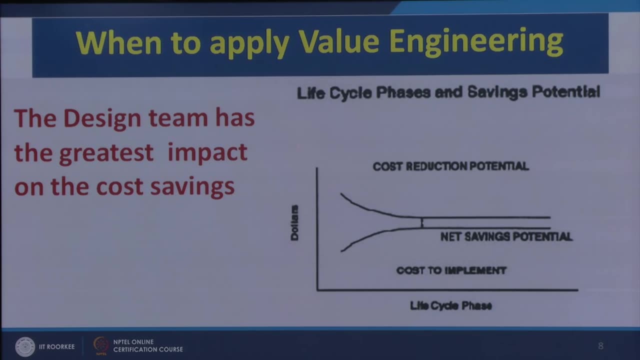 i will address during the course of our discussion. now this is when to apply the value engineering concept. so this i will try to explain briefly. this is the cost in, or the money. this is the life cycle. so if you see, cost to implement the change is increasing and cost reduction. 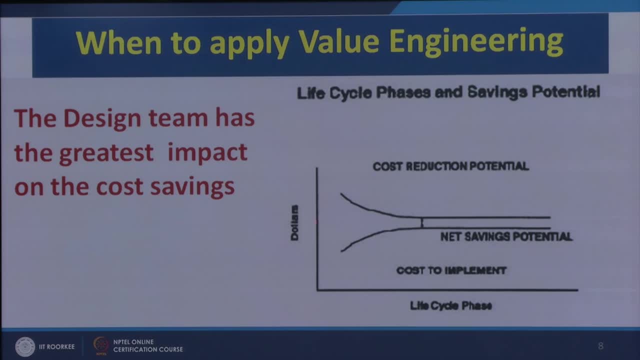 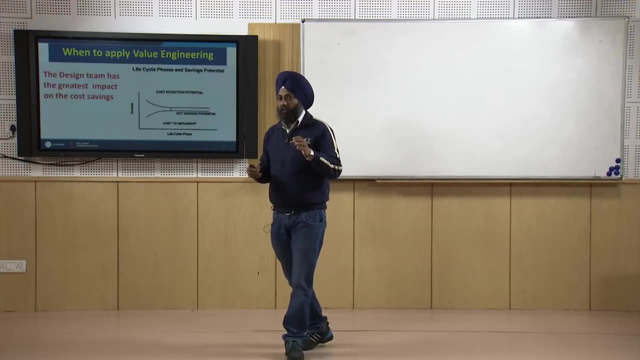 potential is decreasing. so this is the gap here, that is, a net saving potential cost to implement the change. why it increases? because, suppose i am designing a product. my product design is on my screen. for example, if i am using a software, cad software, i have designed a product on my screen. if slight modification is required immediately, i will change the. 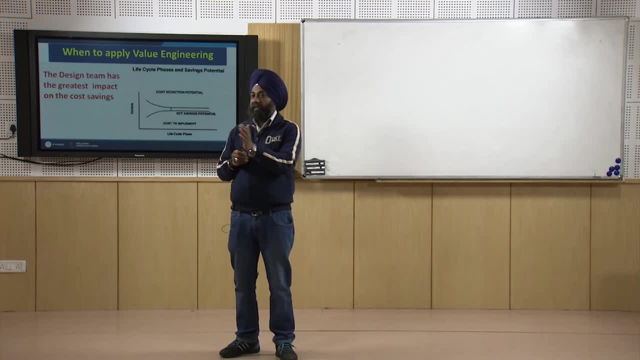 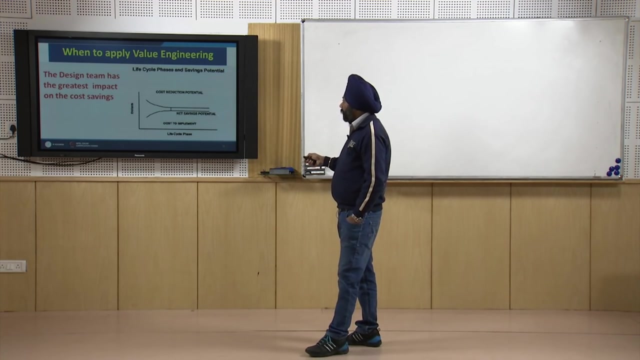 file and will not cost much, but suppose it has already been prototyped. some ah- you can say ah- models have already been made and test marketing is going on. at that stage, if i change, what will happen? the cost to implement will keep on changing and similarly the cost reduction. 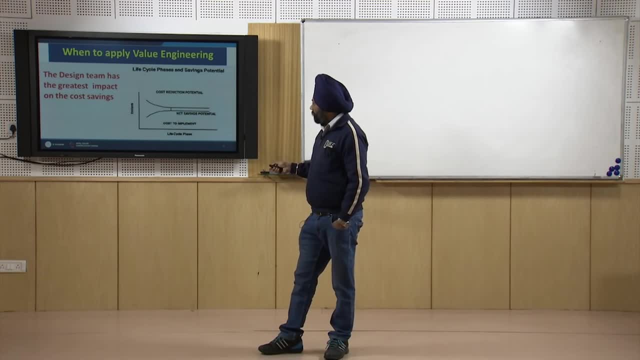 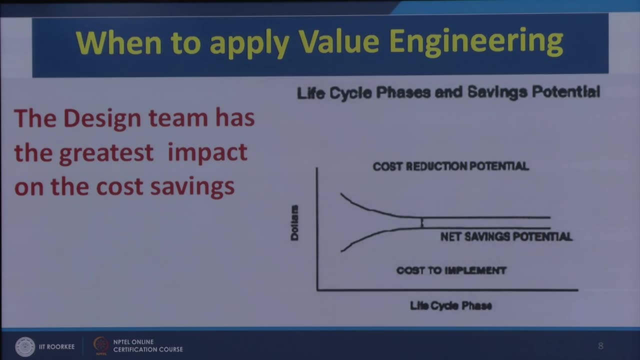 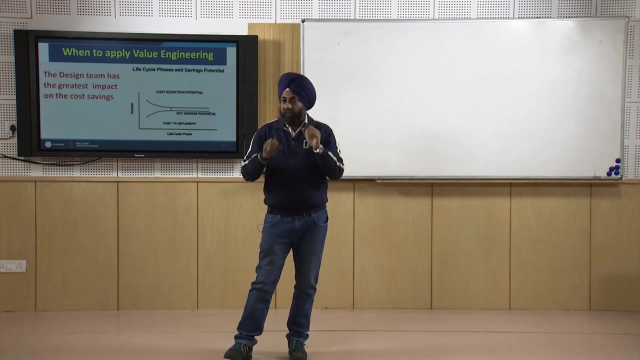 potential will keep on reducing. so it is always evident that we should apply the concept of value engineering in the very beginning stage only, or at the design stage only. ok, so the design team has the greatest impact on the cost saving and, if you remember, in one of the previous classes we have seen that the cost is logged at the design stage seventy. 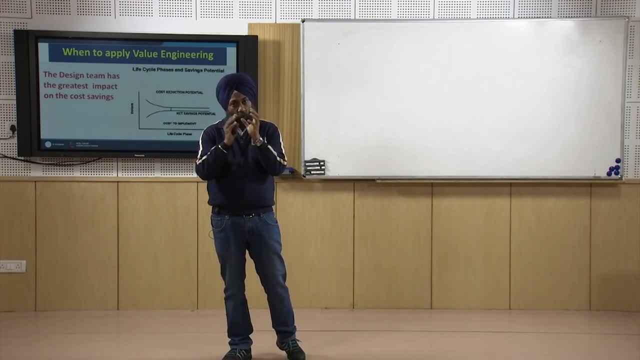 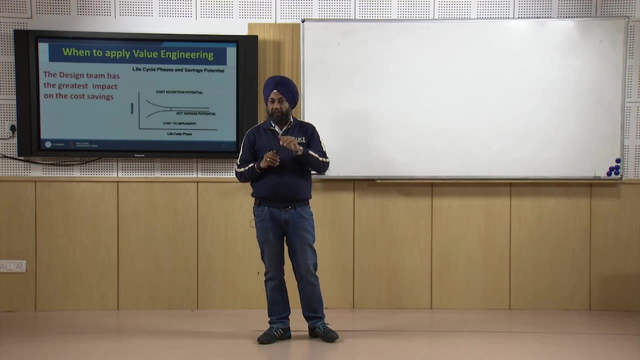 to eighty percent of the cost of the product is logged or freezed or finalized at the design stage. only only twenty to thirty percent of the cost is may be ah controlled during the manufacturing stage. so it is always important. since this technique is related to the cost aspect of the product, it is important to apply this. 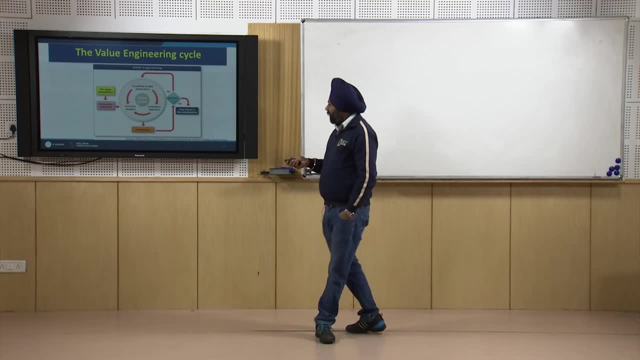 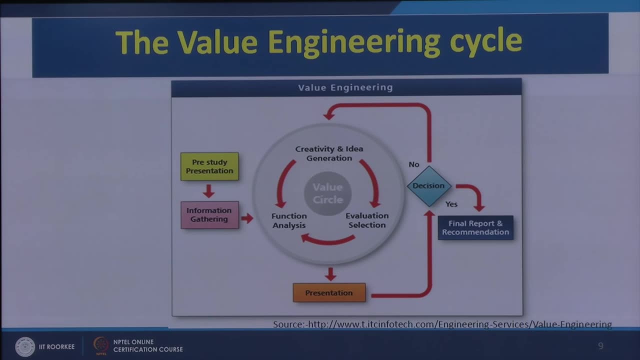 technique at the design stage only now. this is a typical value engineering cycle. it is ah given if it at google. if you ah type value engineering cycle, you will get this diagram so very quickly. i will just go through this. maybe we will come to this again in the 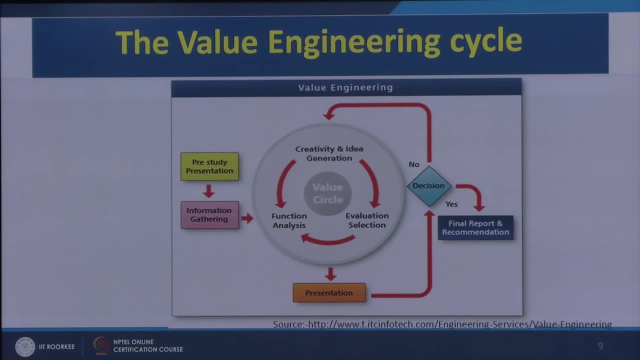 next lecture there is a pre study, presentation, information gathering, and then this is the main value engineering cycle. this is common to any engineering technique use. you have to do a pre study, then you have to collect the information, but this is the main value engineering cycle, that is. 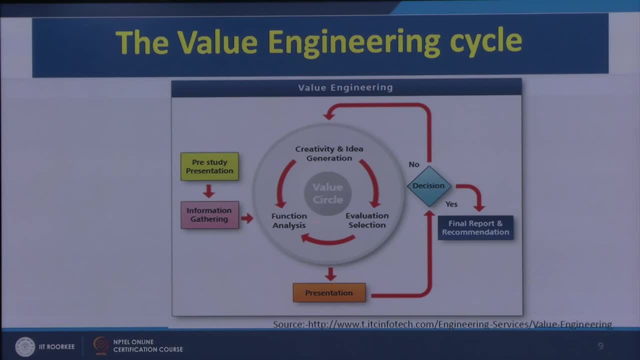 creativity and idea generation, functional analysis, evaluation and selection in order to solve any problem. these are the three things and then finally, there is a presentation. if the ah ah solution is acceptable, next stage, final report, not acceptable, again it goes into the circle again. you create, innovate, generate new and new ideas, do the functional analysis with those ideas and finally do the. 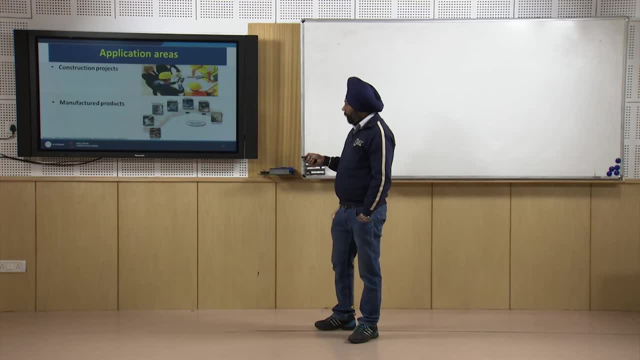 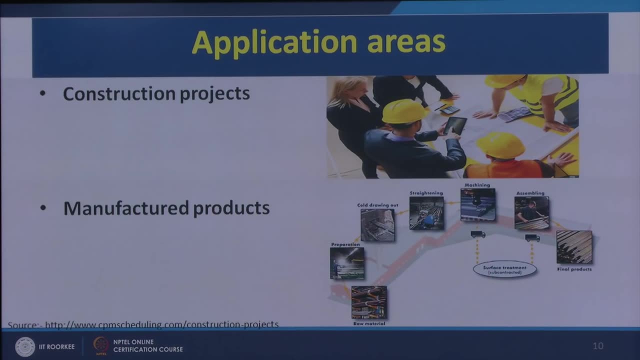 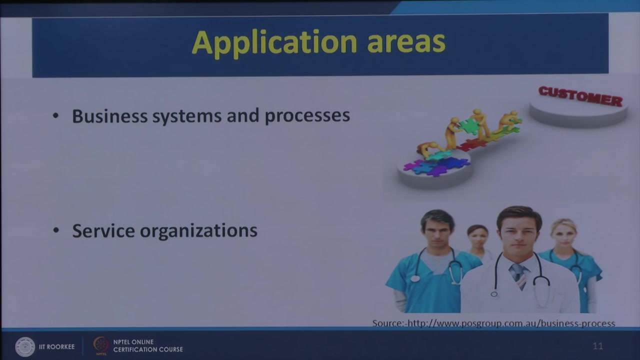 evaluation and selection. so the application areas of value engineering construction projects is one area. manufactured, product or manufacturing is going on. any product which is being manufactured is a may be a computer screen or a computer cpu. anything that is manufactured is, can be, can use value engineering concept, business systems and processes. 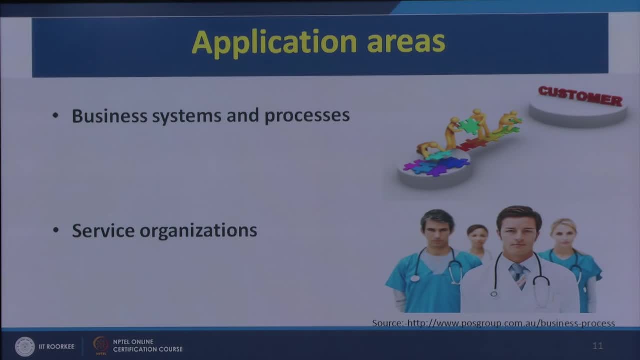 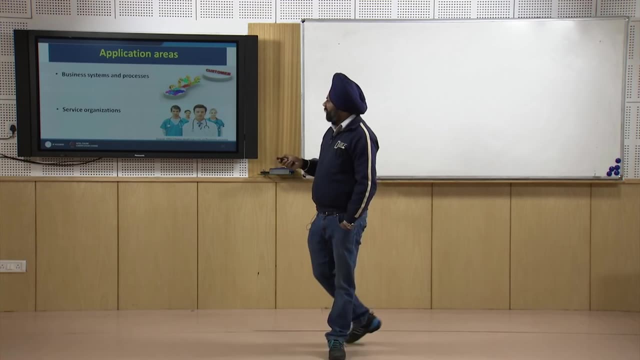 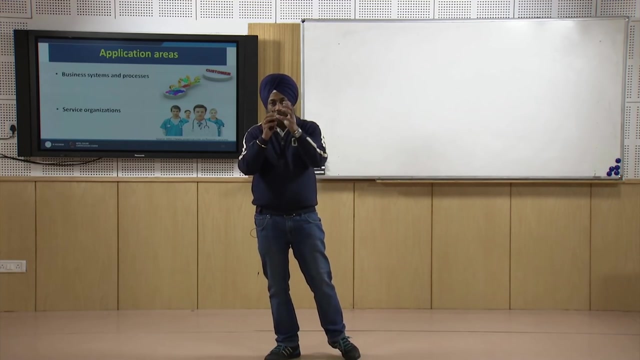 can also use service organizations like hospitals, airports, ah hotels. all these industries can use the basic concepts of value engineering. so we can say that this is ah the application. so application is not only limited to the tangible process products, it is limited to the service industry also. so may be. i will stop here in for todays. 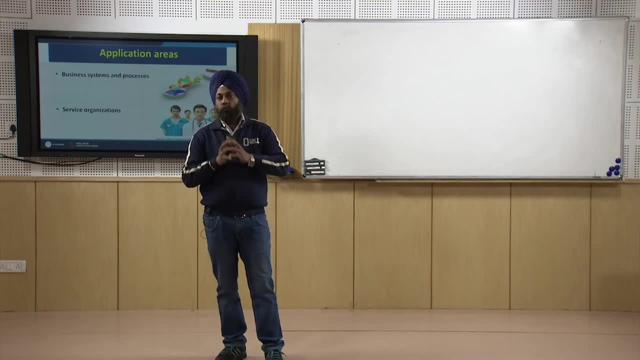 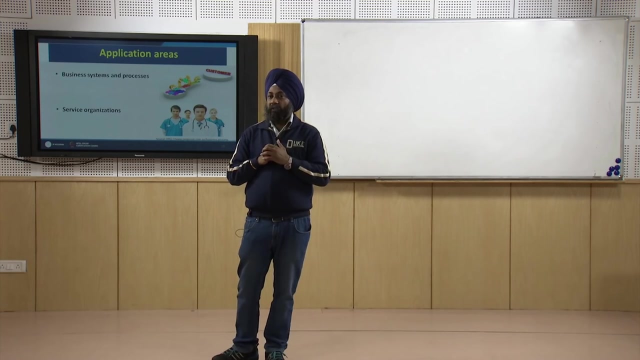 lecture. we have seen today the basic concept of value engineering, the basic concept of function. we will discuss the functions again in the next section and try to relate it with the product design. so we have seen the basic concept of value engineering, the definitions of value engineering and some myths or some misinformation that value engineering is similar. 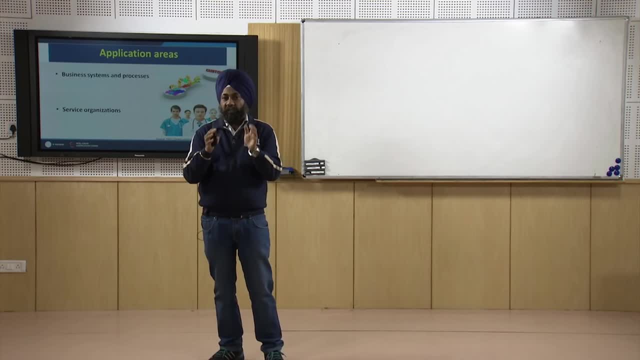 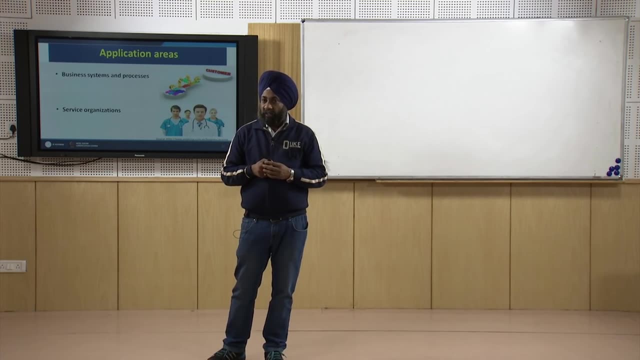 to cost category. we have tried to address that. value engineering is not cost cutting or a design review process. it is a entirely different technique. it is a systematic technique and which can be applied to different application areas, that is, it can be applied to design of new products. it.